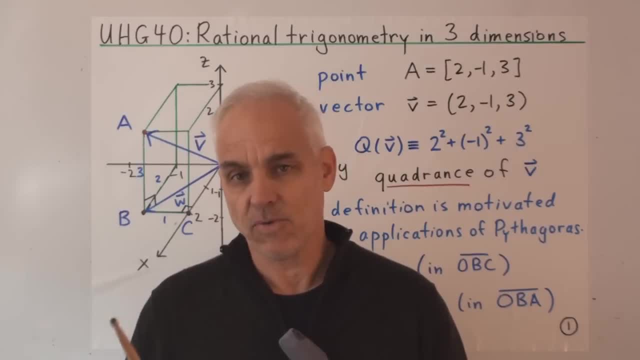 situation. The approach that we've been taking is a vector space approach, where the dot product or inner product or scalar product plays a kind of foundational building role And quadrants and spread are ultimately very strongly connected with this dot product. This is a very flexible and useful approach because it allows us to extend things to higher dimensions. 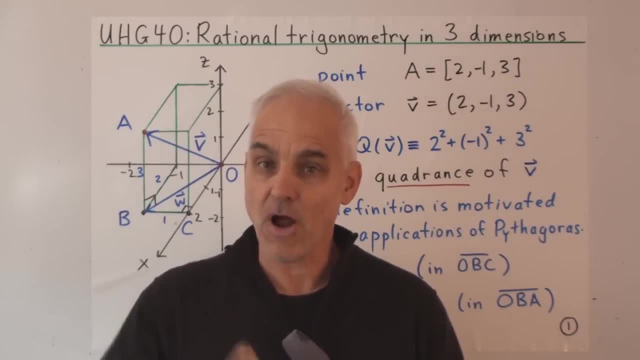 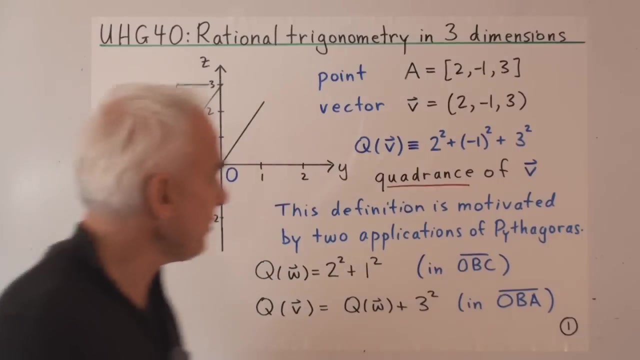 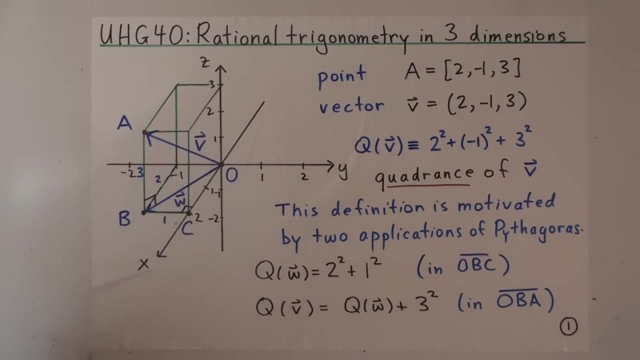 relatively easily And, as we'll see later on, it also allows us to extend things to other kinds of inner products, like relativistic inner products, with a minimal amount of change. So we're working in three dimensions today. Here are the familiar three axes: X axis coming out at us, Y axis, Z axis in the board. 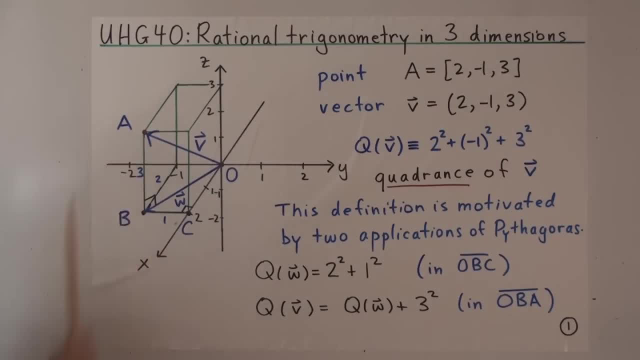 X axis coming out at us. Y axis, Z axis in the board. X axis coming out at us, Y axis, Z axis in the board. A point like this, point A, is denoted by three numbers: x, y and z, coordinates in square brackets. 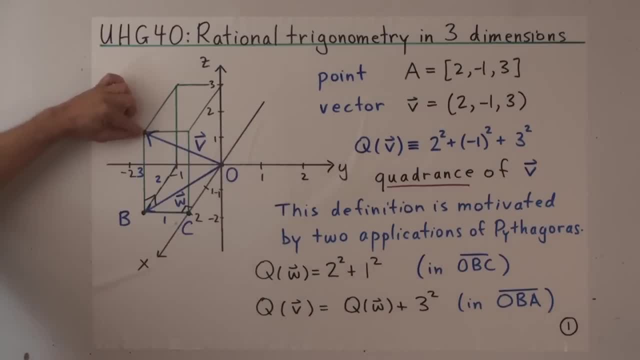 And the 2, minus 1, 3 can be represented physically by going 2 in the x direction, by going minus 1 in the y direction, so that's in that negative direction there, because the positive y direction is there, and going 3 up in the z direction. 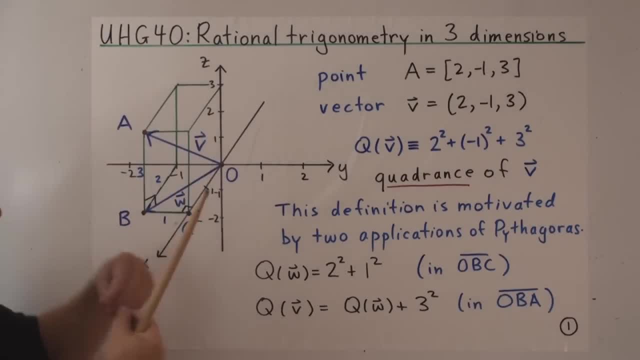 And then we can use those three different extents along the three different directions to make a box or, more fancy term, a parallelepiped That gives us a three-dimensional understanding of where exactly this point 2, minus 1, 3 is. 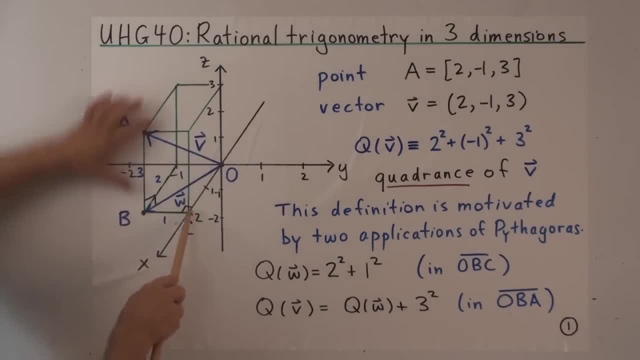 So 2, minus 1, 3.. It's that box there and it has sides: 1 in this direction, 2 in this direction and 3 in the vertical direction. Associated to that point is a vector, and we can think of this vector as being the vector from the origin O to the point A. 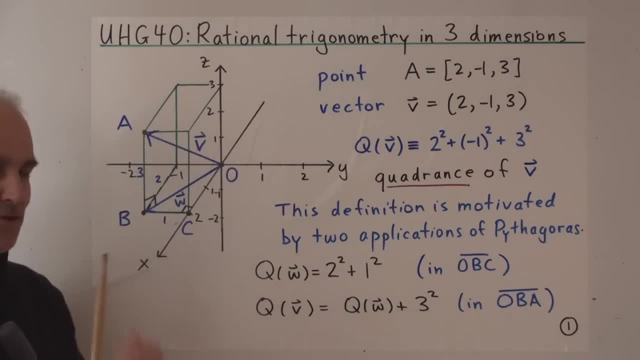 So the vector is this directed line segment between the two points, And it's given by the same triple of numbers in round brackets. And then the fundamental metrical concept is that of the quadrants of the vector. The quadrants of this vector is the sum of the squares of the coefficients. 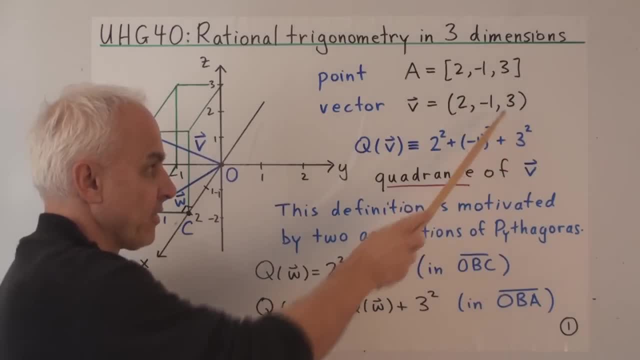 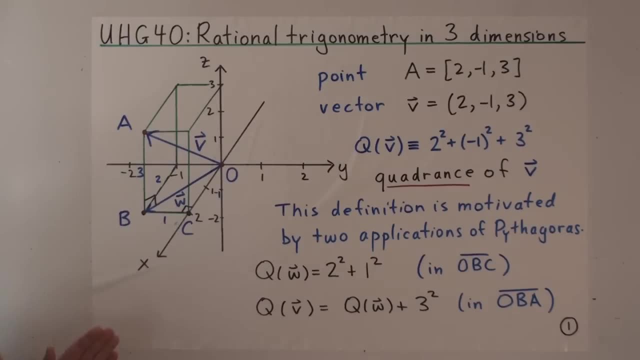 2 squared plus minus 1 squared plus 3 squared, So that would be, in this case, 14.. Now, this definition is motivated by two applications of the planar Pythagoras' theorem, So there's a reason why we choose this. 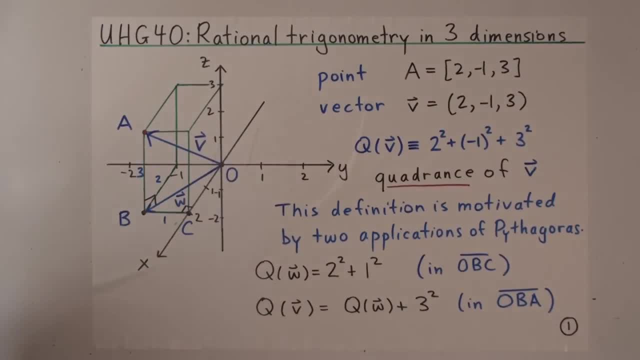 We choose this particular combination and not something else, And we can understand that in this picture by getting to this vector in two steps. First of all, let's think about this vector W, which is the projection of V onto the xy plane. So this is a vector whose x coordinate is 2, and whose y coordinate is minus 1.. 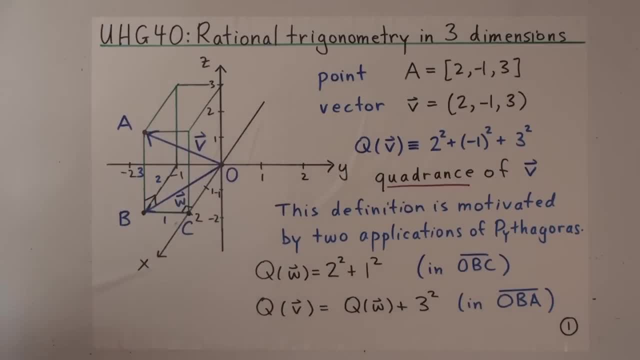 There, it is right there. It's in the xy plane And the quadrants of that vector, according to a two-dimensional Pythagoras, would be 2 squared plus 1 squared. So once we've got the quadrants of this vector, 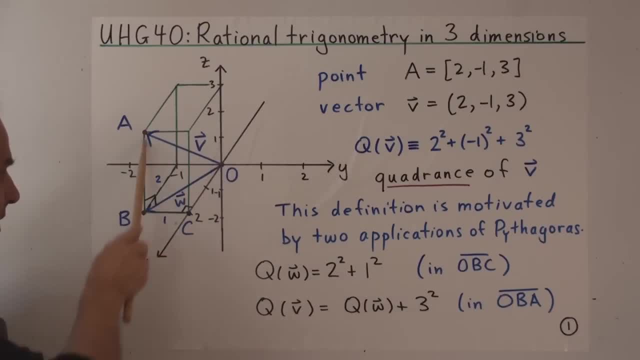 then have a look at this triangle here, the triangle OAB, which is also a right triangle. So that's a right triangle because this vector here is in the z direction That's exactly perpendicular to to the xy plane. So there's a right angle there. 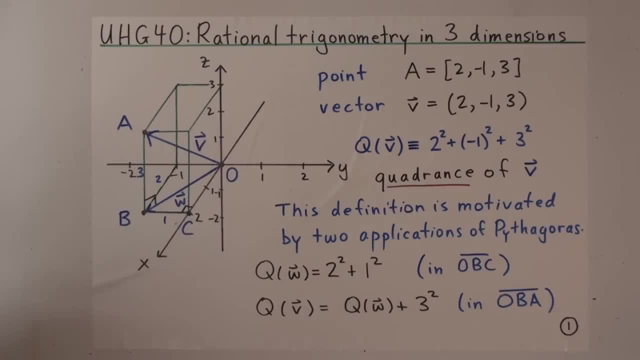 perpendicularity between this line and this line. So now in this planar triangle we can apply Pythagoras again, and this quadrants plus this quadrants equals this quadrants, telling us that the quadrants of V is the quadrants of W plus 3 squared. 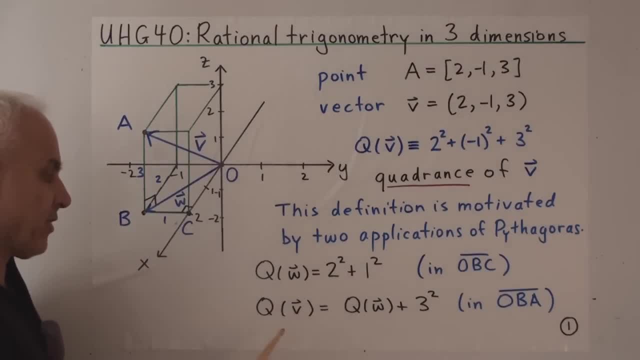 So when we put this one together with this one, we get that the quadrants of V is 2 squared plus 1 squared plus 3 squared. That explains why we're taking the sum of the squares of the three coefficients, And you might just like to convince yourself. 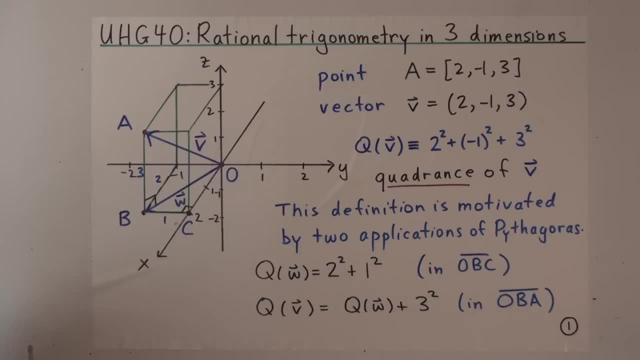 that we could have a similar diagram by projecting V not onto the xy plane but also onto the xz plane, for example, or onto the yz plane, And you can think about where those corresponding vectors and right triangles would be in the diagram. 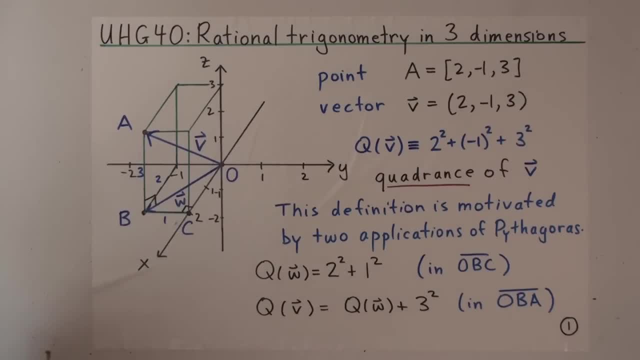 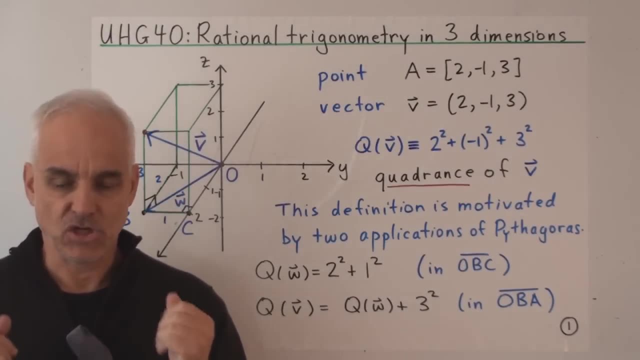 All right. so fundamental idea that the notion of quadrants for a vector in three-dimensional space is the sum of the squares of the coefficients- And this is just Pythagoras- applied twice in two sort of different planar directions, Just as in the planar case. 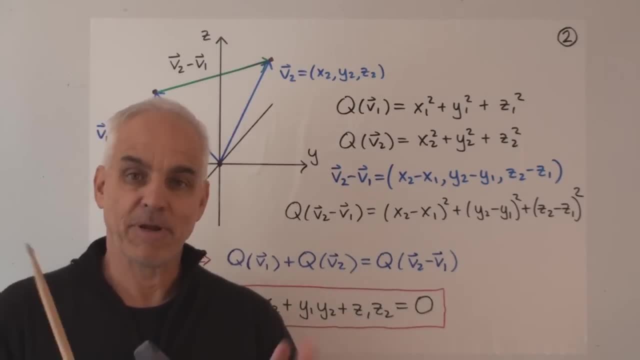 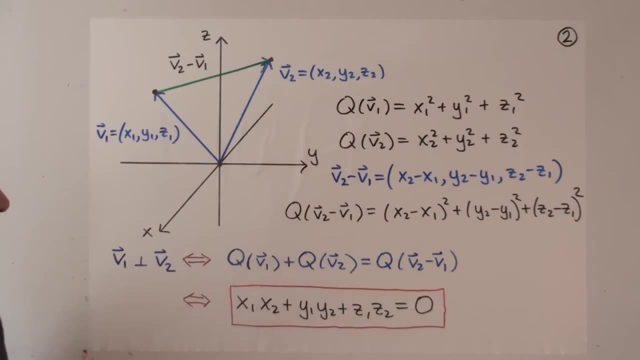 Pythagoras' theorem not just motivates the definition of quadrants, but it also motivates the definition of quadrants. It also explains to us how to understand perpendicularity. So here we have two vectors, V1 and V2.. The coordinates of V1 are x1, y1, z1.. 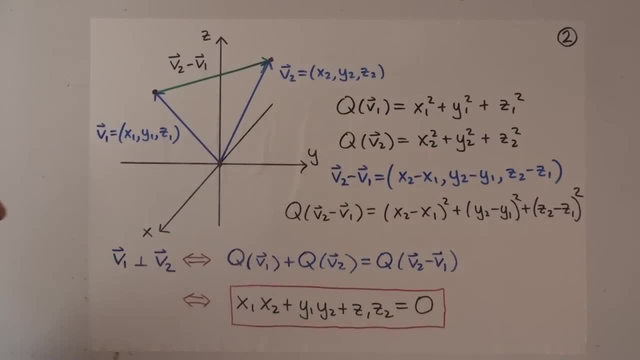 The coordinates of V2 are x2, y2, z2.. Here's the quadrants of V1, and here's the quadrants of V2.. Another vector that's interesting is the vector from here to here, The difference between the coordinate V2 and the coordinate V1. 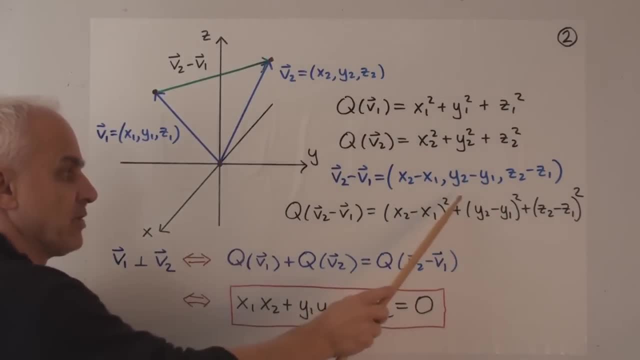 So V2 minus V1 is this vector here x2 minus x1,, y2 minus y1, and z2 minus z1.. And here is its quadrants. So Pythagoras' theorem applied to this triangle says that these two lines here are perpendicular. 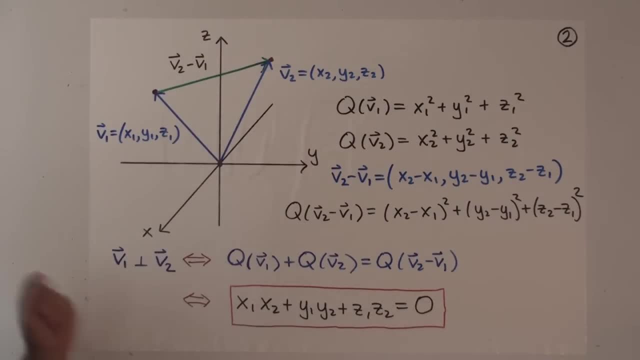 So we have a right angle there, precisely when this quadrant plus this quadrant equals this quadrant. So V1 and V2 are perpendicular precisely when Q of V1 plus Q of V2 equals Q of V2 minus V1.. So if you look at this equation, 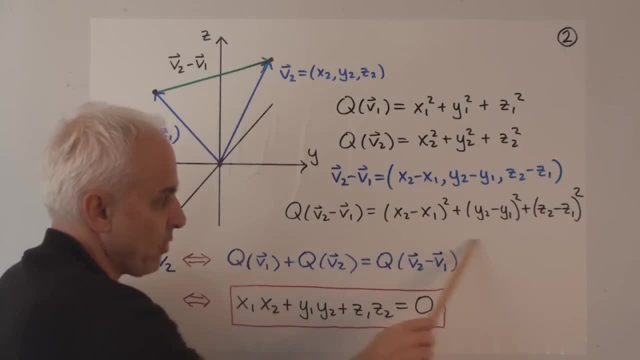 there's Q of V1, there's Q of V2. If we set that equal to this, then we can expand this out and cancel the common term and we can cancel the common terms on the left-hand side. In fact, all of these terms will be cancelled out. 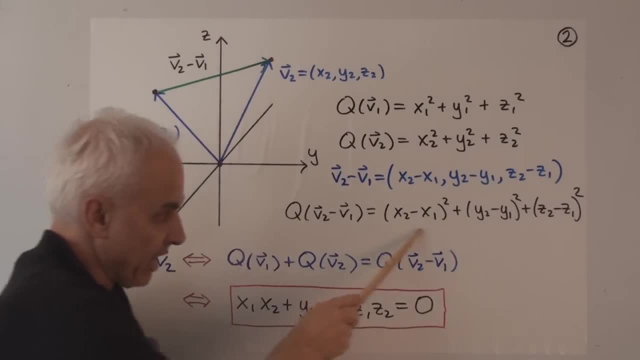 with the corresponding term on the right-hand side, And the only thing we'll be left with on here is minus 2x1, x2 from here, plus minus 2y1, y2 from here, plus minus 2z1, z2 from here. 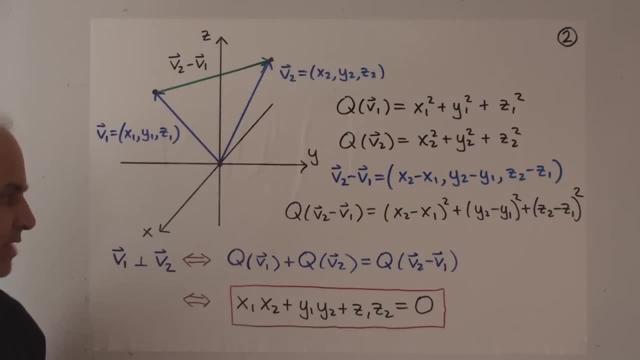 So that'll all be equal to zero. That's what this equation comes down to. So remember, if we multiply by minus 1, divide by 2, then we are getting this relation: x1, x2, plus y1, y2, plus z1, z2 equals zero. 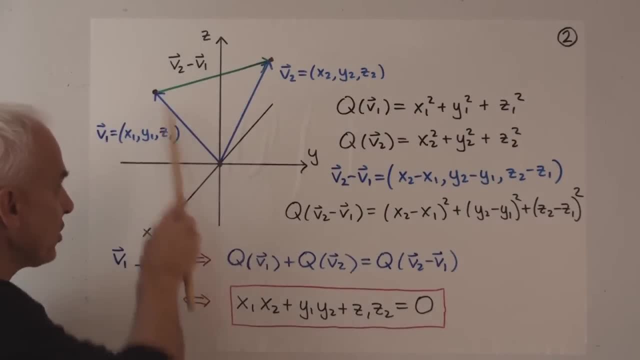 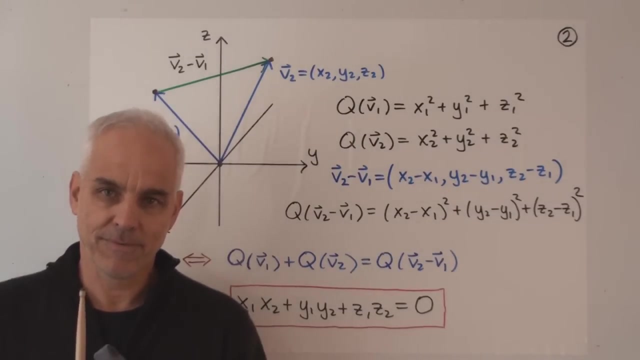 So Pythagoras' theorem tells us that these two vectors are perpendicular precisely when this particular relationship is satisfied between the coefficients of the two vectors. This is where the dot product comes from. The dot product is not just something we make up, It is a consequence of Pythagoras' theorem. 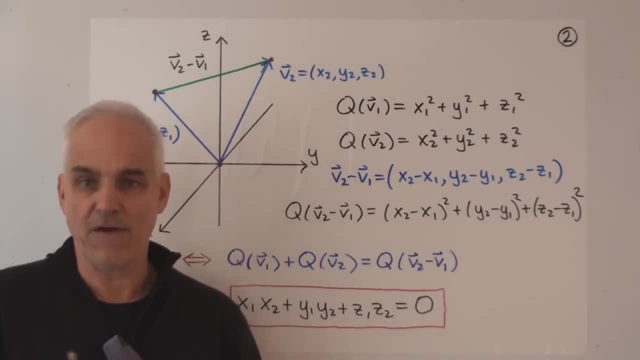 Unfortunately, students taking linear algebra courses are not told this often. This is not stress, but it's very important to understand this. The dot product is coming from Pythagoras' theorem. It's the number one theorem in mathematics. This is a manifestation of it. 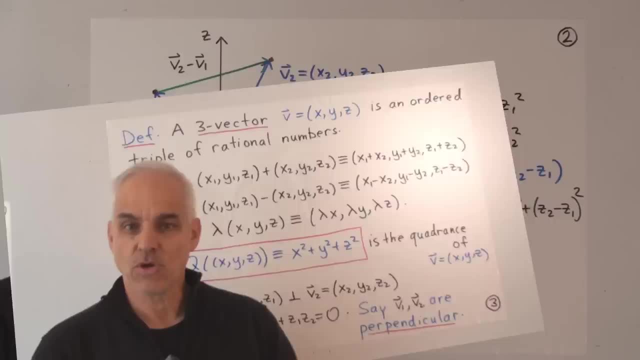 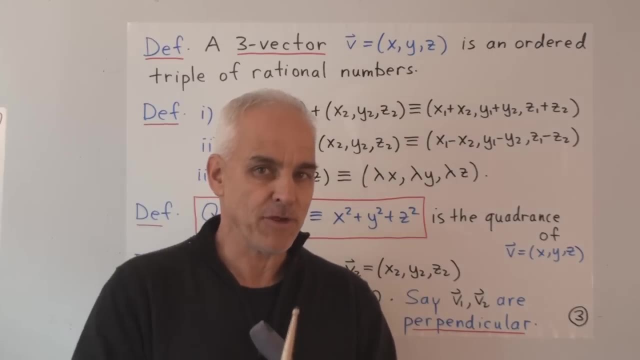 in terms of coordinates. So we should think of all of that as being motivation, Just as in the planar case, we are happy to be motivated by Euclidean geometry, but we do not want to rest our theory on that as a foundation. 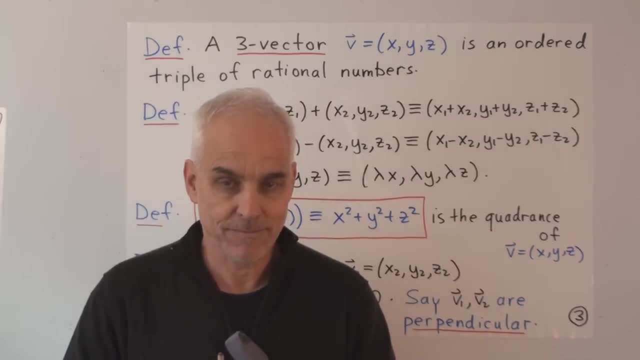 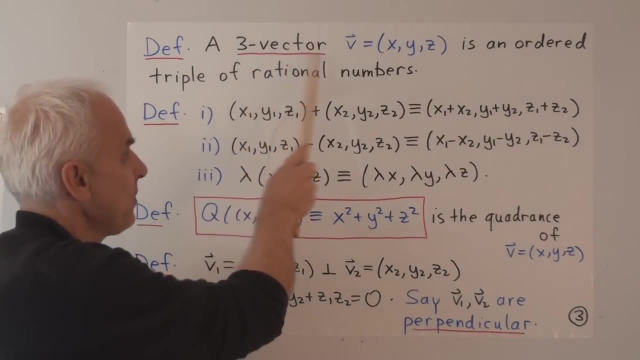 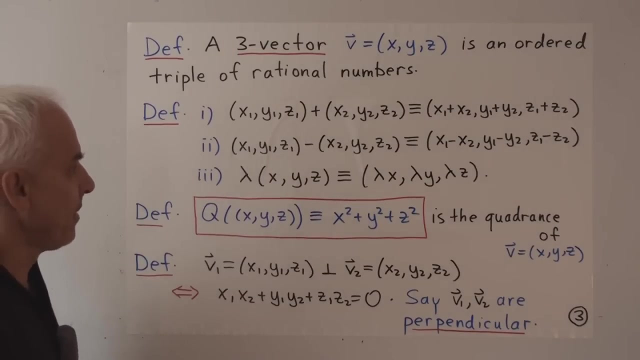 because there are problems with Euclidean geometry. So we start with our definitions from scratch. A three vector now is a triple, an order triple of rational numbers: x, y, z. A three vector now is a triple. I will often say vector instead of three vector. 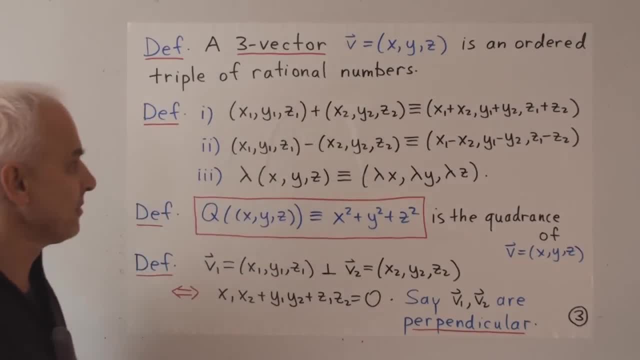 if the situation is obvious what I'm talking about. So here is how we add two vectors, just component-wise. Here's how we subtract two vectors, component-wise. Here's how we multiply a vector by a scalar, again component-wise. 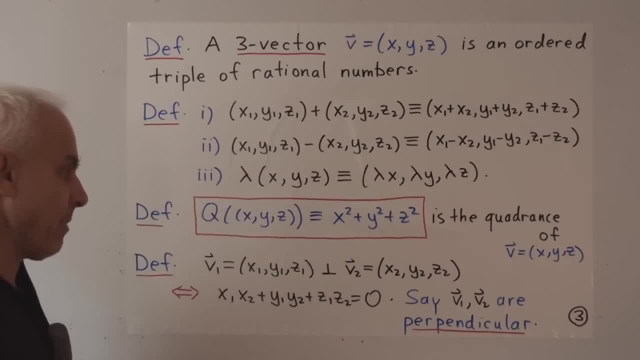 Here's our definition of the quadrants. That's motivated by our previous discussion, but you can just say this is just a definition that we rather arbitrarily make In this purely algebraic context. That's the quadrants of the vector x, y, z. 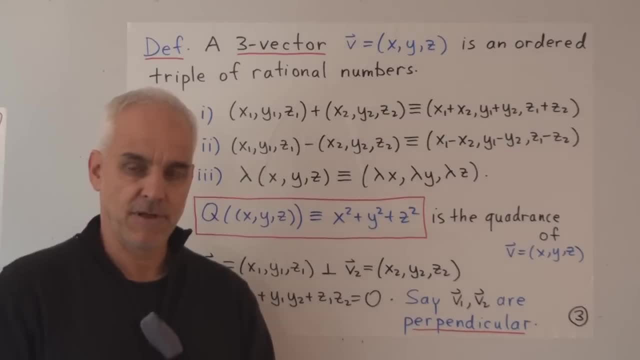 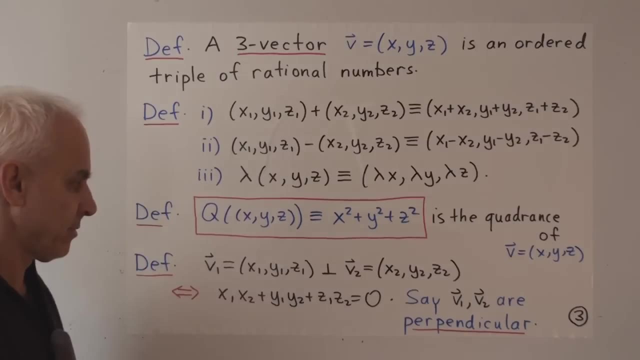 And then we define the perpendicularity of two vectors. We say that two vectors are perpendicular precisely when this relationship holds. Again, that's motivated by the previous discussion, but it's logically independent of it. We're just defining this as the quadrants. 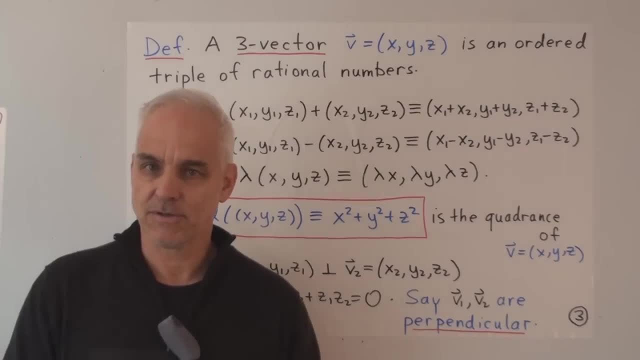 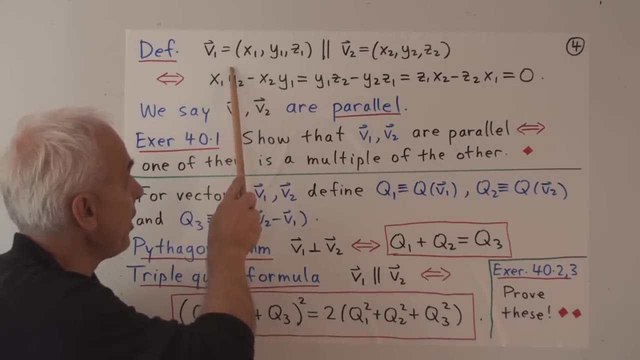 We're defining this as perpendicularity of vectors. Now let's introduce the idea of parallel vectors. So two vectors- v1 and v2, are parallel. That happens precisely when this equals 0,, this equals 0, and this equals 0. 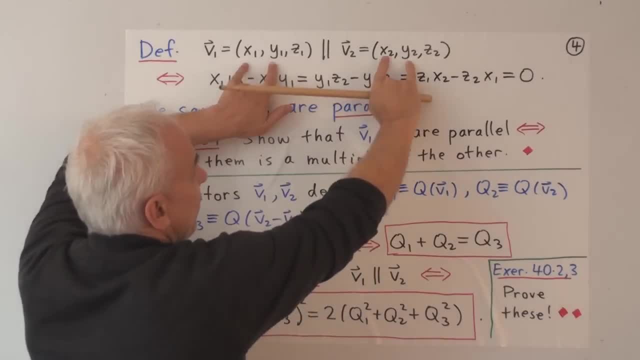 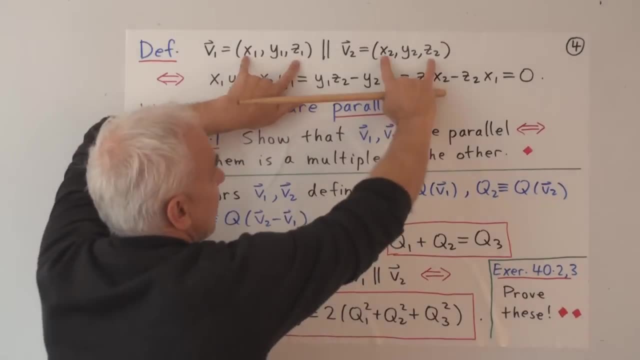 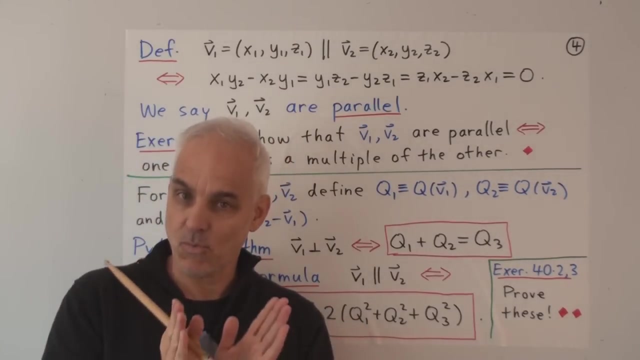 In other words, we require that this pair and this pair are proportional, That this pair and this pair are proportional, That this pair and this pair are proportional and this pair are proportional, and that the x and z pairs are proportional. so, as opposed to the two-dimensional situation where there was simply one equation, that 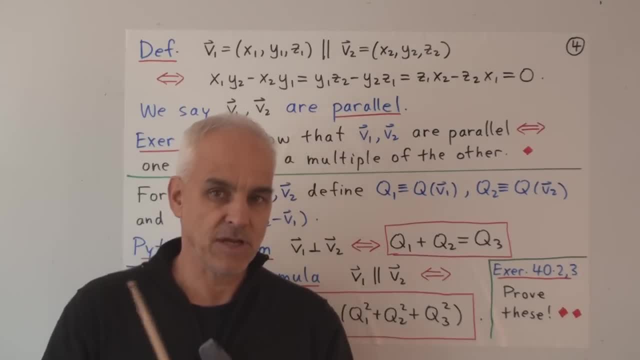 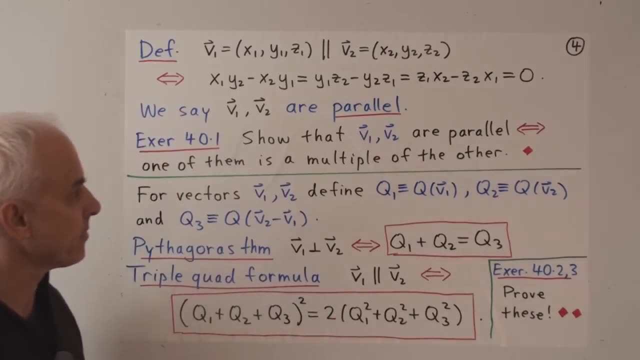 you had to check here. there are three equations that you need to check and in general, you do need to check all three equations. so when this happens, we say that be one in V2 are parallel. good little exercise. convince yourself that this definition really amounts to nothing more, nothing less than saying: 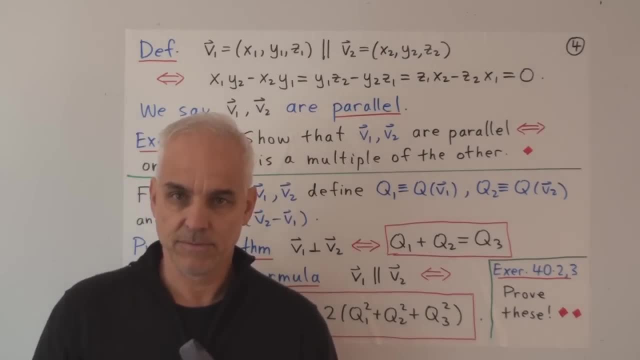 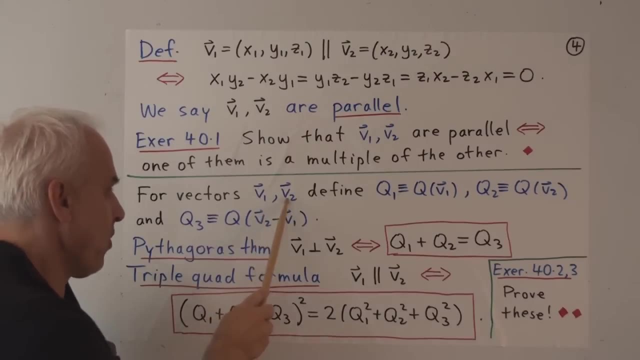 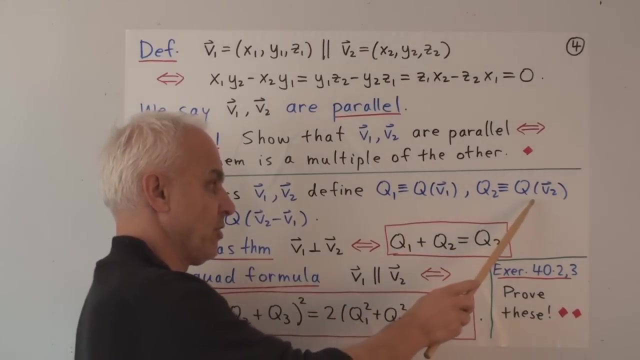 that one of the vectors is a multiple of the other. ok, so now suppose we have two vectors, v1 and v2, and let's define three quadrants: q1 is the quadrants of v1, q2 is the quadrants of v2 and q3 is the quadrants of the difference between the 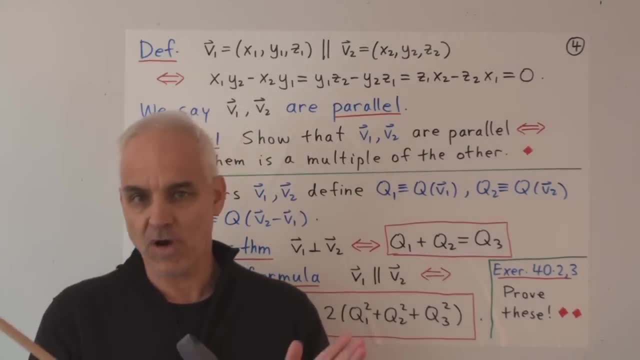 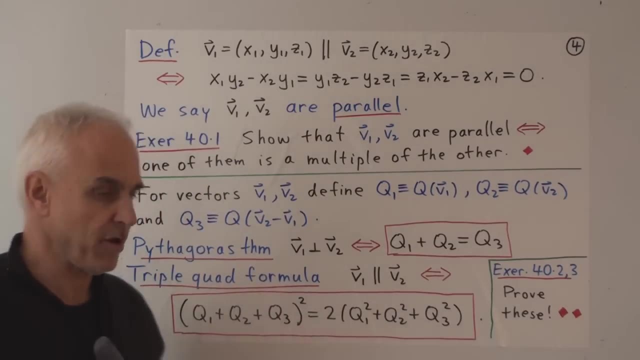 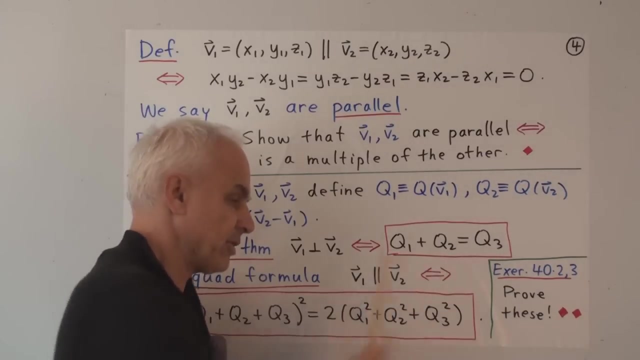 vectors, so the third side of the triangle formed by v1 and v2. here are our two most important theorems: Pythagoras's theorem: v1 is perpendicular to v2 precisely when q1 plus q2 equals q3, and v1 is parallel to v2 precisely. 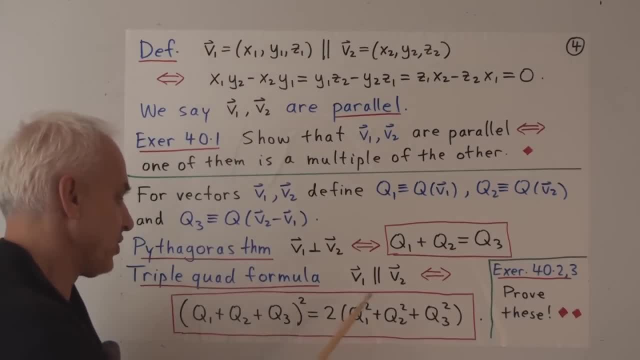 when q1 plus q2 plus q3 squared equals 2 times q1 squared plus q2 squared plus q3 squared, that triple quad formula. again the two most important theorems in mathematics. this one, everybody knows that this one. the year 2012, not a lot of. 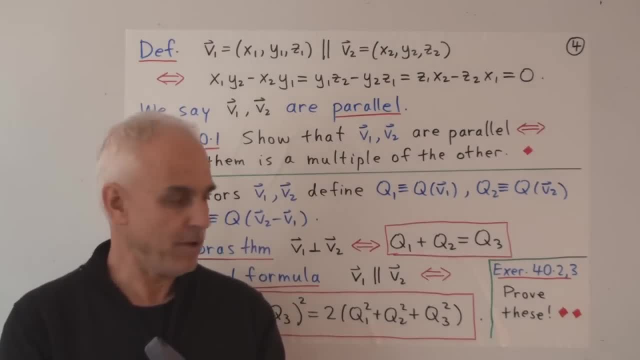 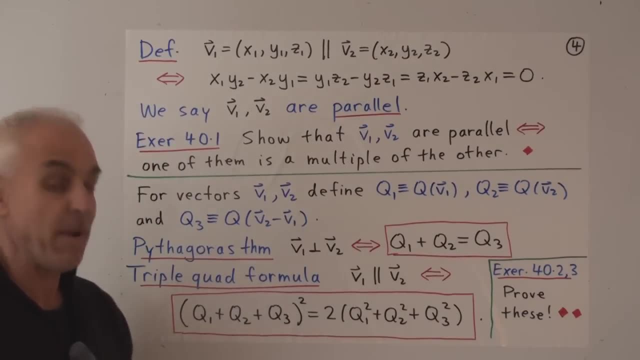 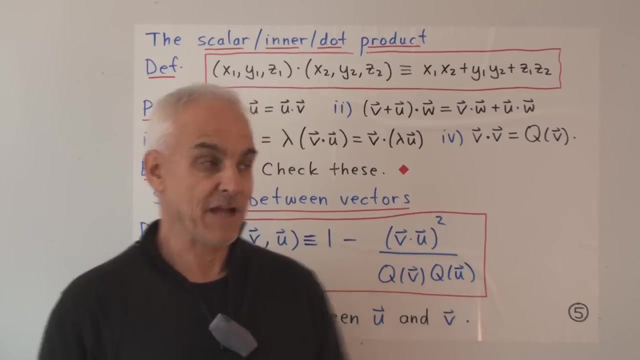 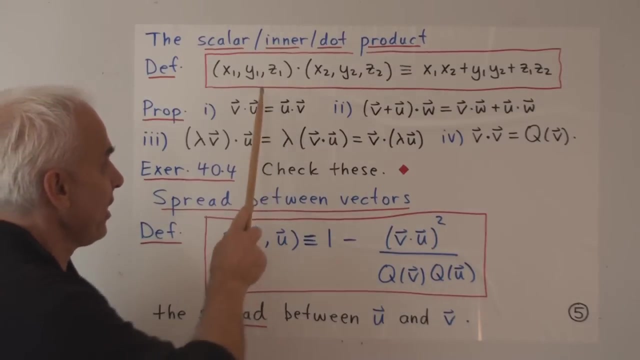 people quite know that yet, but slowly they will so exercise prove these formulas, very parallel of course to our previous lecture. so, again motivated by our previous discussion, we define the scalar or inner or dot product between two, three vectors. in this form the dot product between this three vector in. 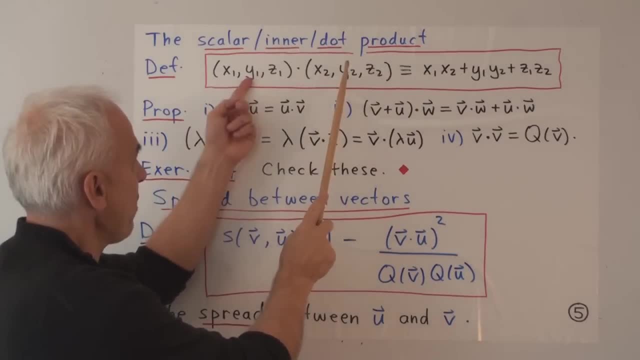 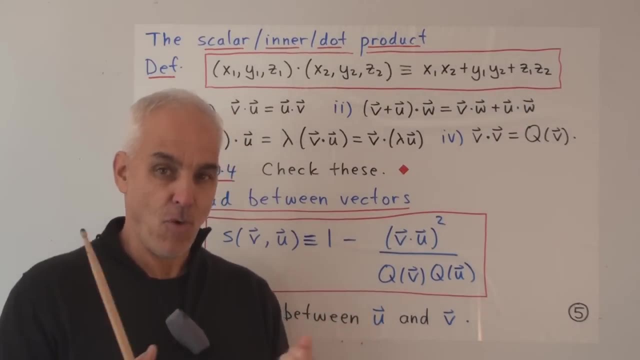 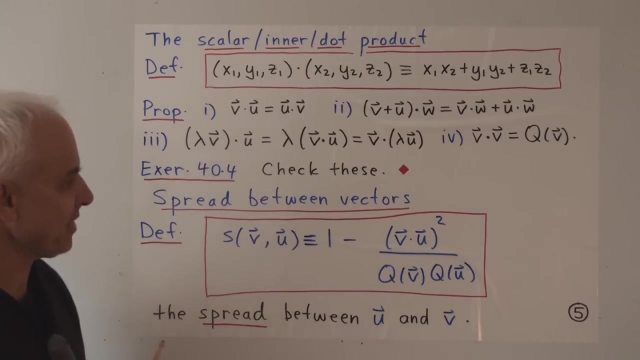 this three vector is x1, x2 plus y1, y2 plus z1, z2. this is some kind of analog of the quadrants formula that applies to two vectors and not to one. so again, exactly as in our last lecture, some obvious, easy to prove aspects of this. 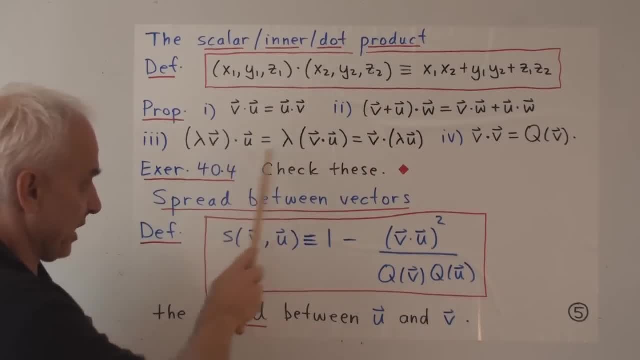 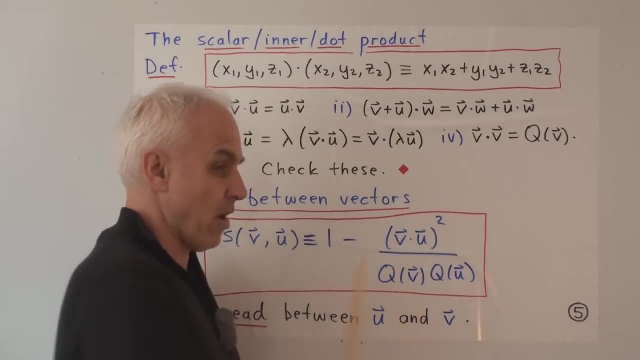 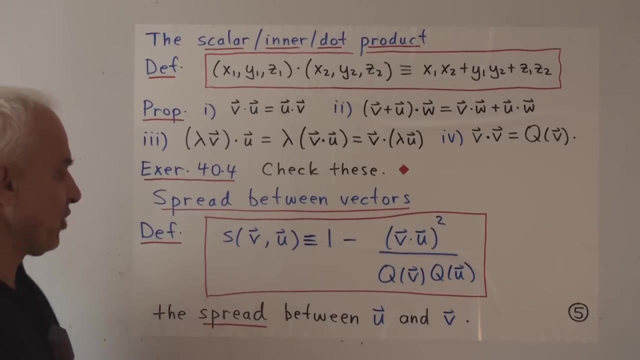 dot product. it's symmetrical, it's linear with respect to addition and scalar multiplication, and when you apply to a vector and itself, you get the quadrants of the vector. please check these. and now the spread between two vectors is exactly the same formula as in the two. 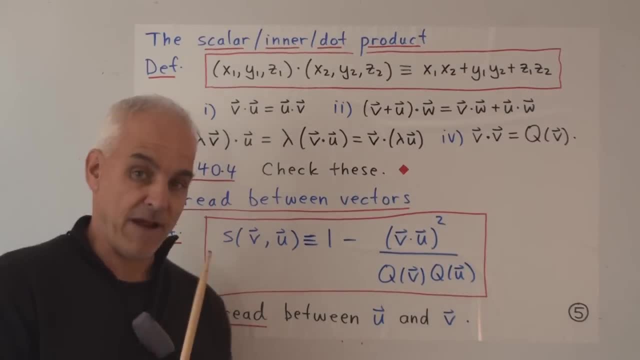 dimensional case, except that now we're talking about three vectors and the dot product here means this three-dimensional dot product instead of the two-dimensional dot product, and the quadrants is the three-dimensional quadrants instead of the two-dimensional quadrants. but conceptually it's exactly. 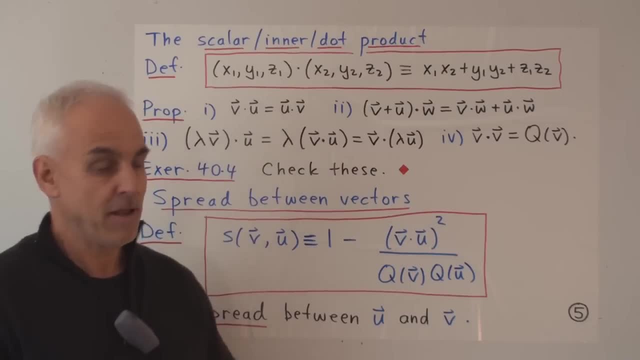 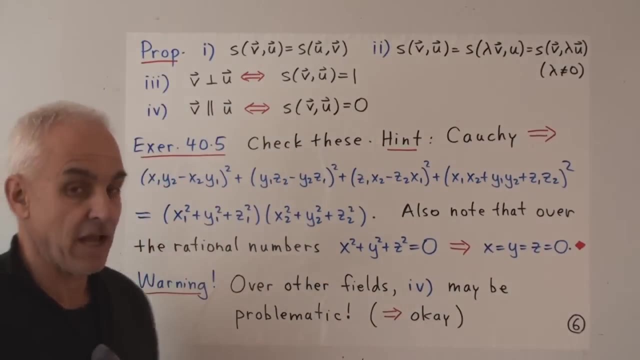 the same formula and arithmetically it ends up working the same. now here is a proposition that records the various elementary properties of the spread. the spread is symmetric. if you interchange the order of the two vectors, the spread doesn't change its invariant. under scaling, you multiply one or both of the vectors by a nonzero number, positive or. 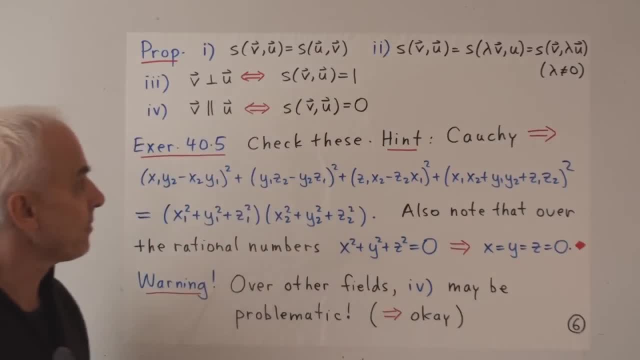 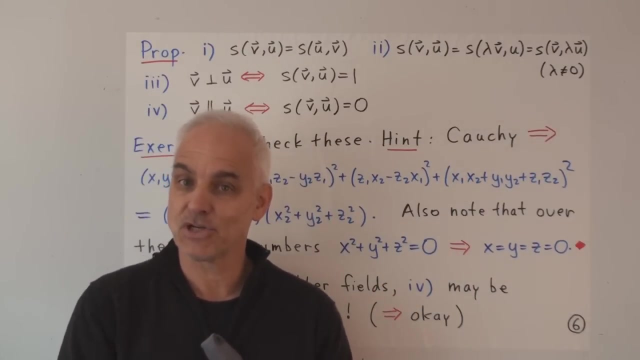 negative, the spread doesn't change. perpendicular vectors have a spread of one and parallel vectors have a spread of zero. so our next exercise: please check these four properties. the first three are routine. the fourth one requires again some more thinking and an important identity due to Cauchy, famous French mathematician of the 19th century. 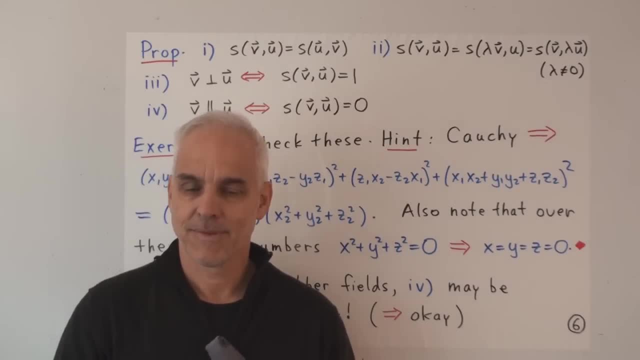 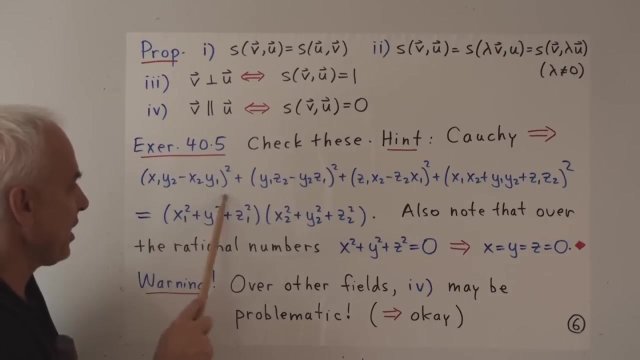 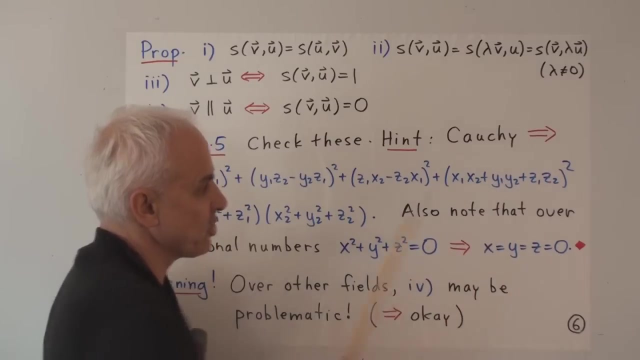 is important for this problem. For this one, the identity is a three-dimensional version of the Fibonacci identity that I mentioned last time, but it's significantly more complicated. it has three of these sort of cross terms all squared plus the dot product expression. squared equals quadrants- kind of term here. times quadrants term here. 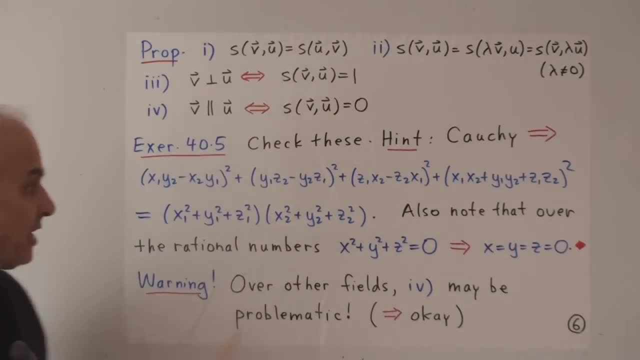 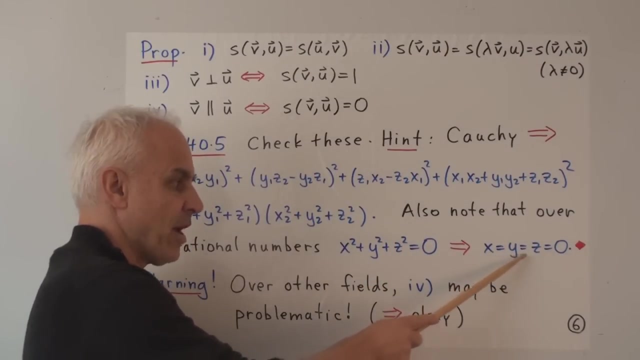 so please check that this identity holds, and that will be useful to prove this fourth property. it will also be perhaps useful to note that, when we're talking about the rational numbers, the equation x squared plus y squared plus z squared equals 0 has only one solution, has a solution: x equals y equals z equals 0. so 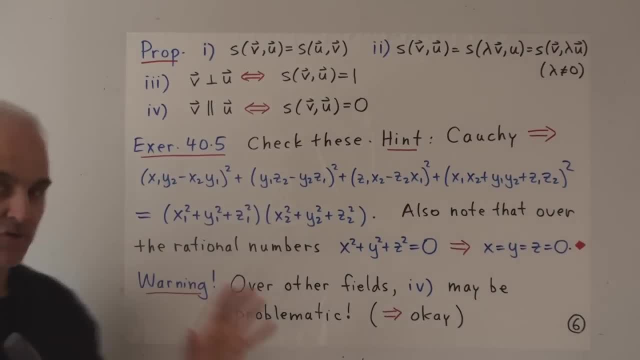 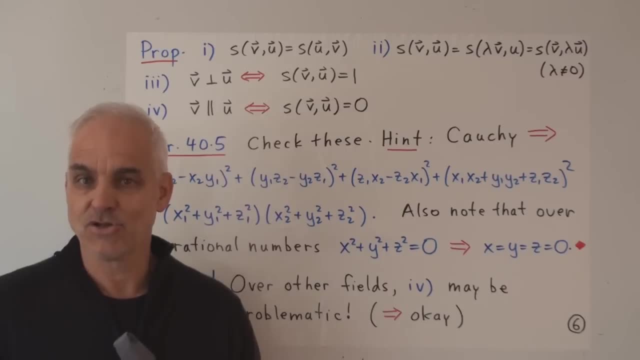 a little bit of a warning. this rational trigonometry that we're talking about now, we're only talking about it over the rational numbers, but in fact it extends to more general fields. but just note that this fourth property does not necessarily extend to more general fields, because this corresponding fact here is not. 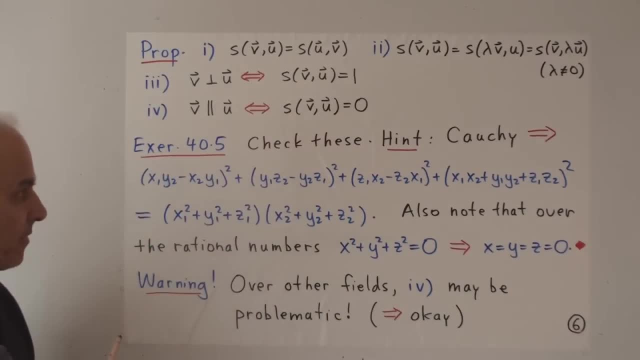 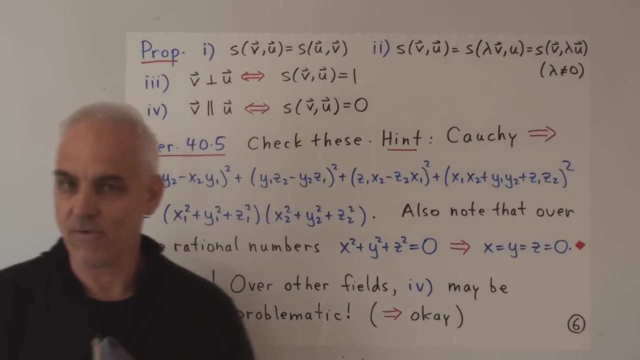 necessarily valid for a general field. so this relationship does in fact work, but this relationship doesn't necessarily hold for a more general field. if you're not familiar with more general fields, don't worry, we'll be talking about those at some later time. and so now we come to the other three main laws of rational. 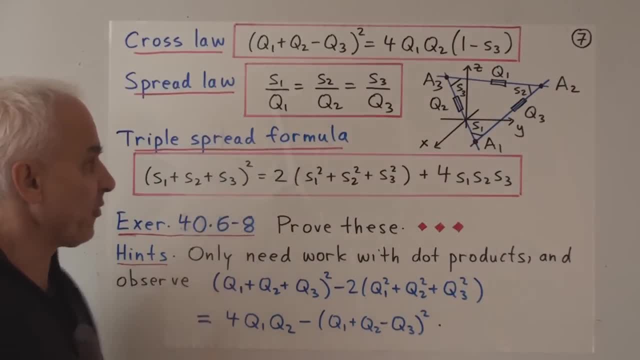 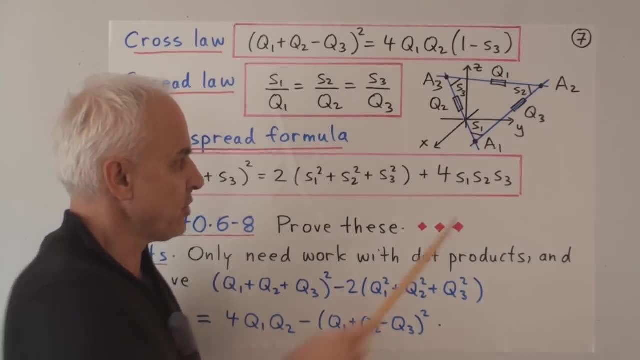 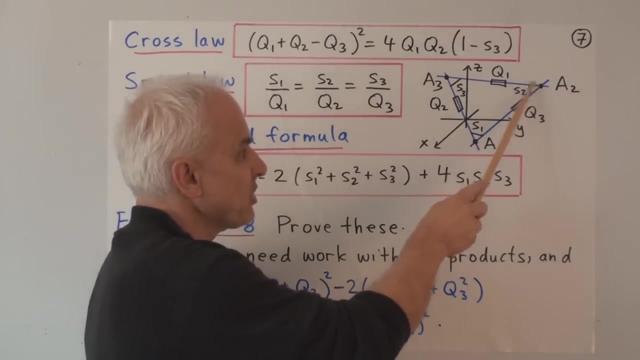 trigonometry, the cross law, the spread law and the triple spread formula, which concern a general triangle in three-dimensional space. so, given any three points- a1, a2, a3- we have three lines. we have three quadrants: is q1, q2, q3 and 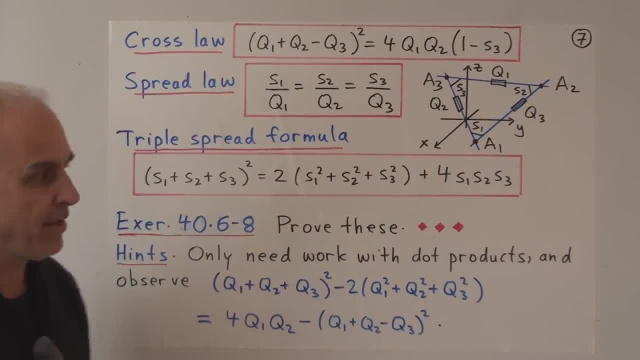 three spreads- s1, s2 and s3- and then the relationship between those six numbers is exactly the same as it is in the planar case and, as an exercise, prove these. so again, you only need to really work with the dot products and again this same relationship. 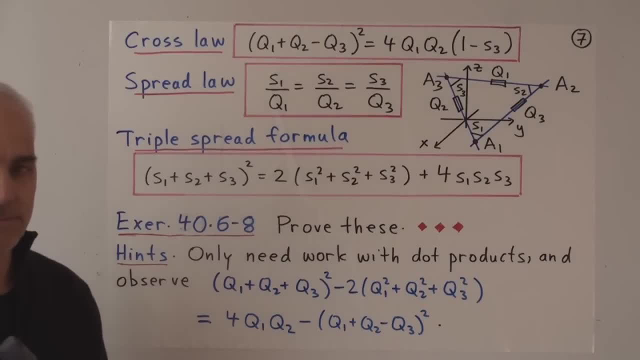 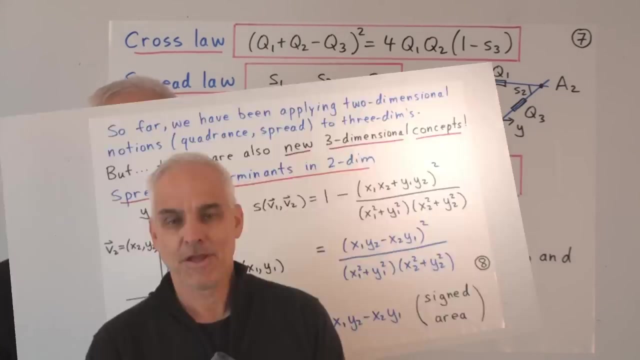 that we've already talked about, is, is useful when it comes to a triangle, the. the laws of rational trigonometry are exactly the same in three dimensions as they are in two dimensions. that's what we're saying here. so is three-dimensional trigonometry pretty well the same as two-dimensional trigonometry? no, it's not. 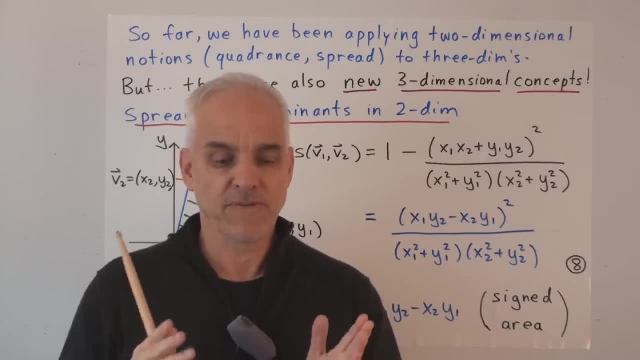 far, far from it. what we've established so far is that the study of a triangle in three dimensions is pretty well the same as the study of a triangle in two dimensions. that's what trigonometry is. in two dimensions is a study of a triangle sort of our basic shape, but in three dimensions a triangle is not the. 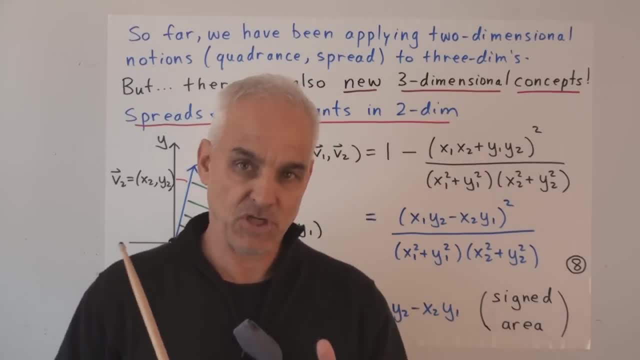 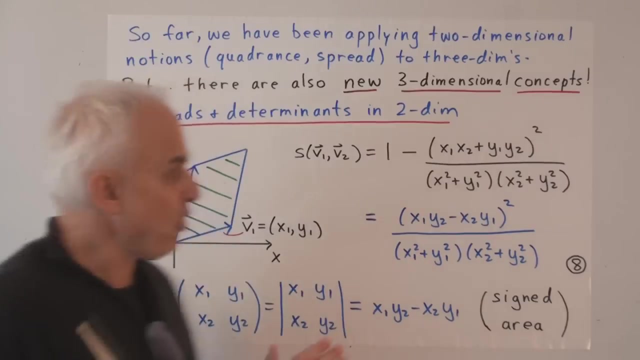 general object. it's not the fundamental object which you want to understand. and in three dimensions there are some other concepts, some slightly more complicated concepts that are necessary to understand trigonometry in this setting. so to motivate that, let's have a look at spreads and determinants in two dimensions. let's go back to the two-dimensional situation and 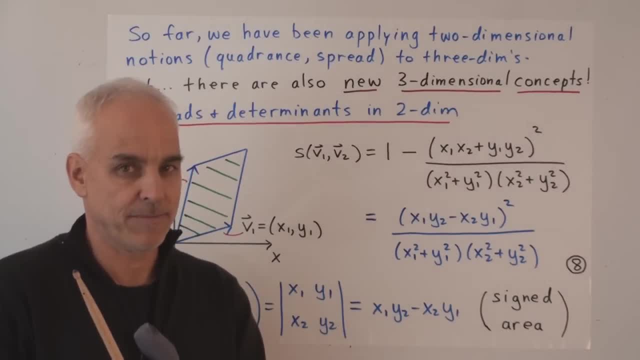 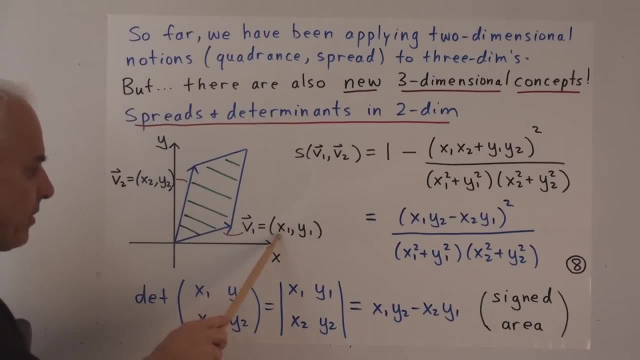 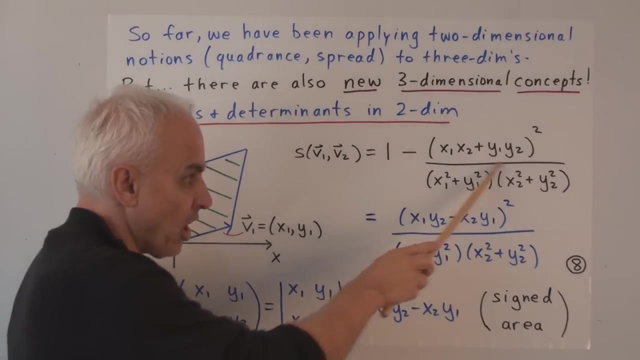 look at the spread in a slightly different way. so here's two dimensions again. here's a two-dimensional vector, v1, which is x1, y1, and here's another two dimensional vector, v2, with coordinates x2 and y2, and here's our definition of the spread between v1 and v2. so it was 1 minus the 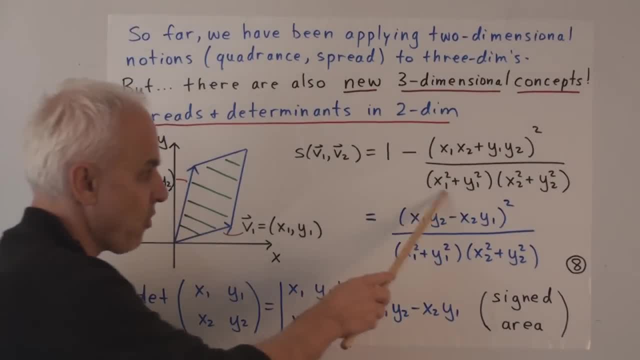 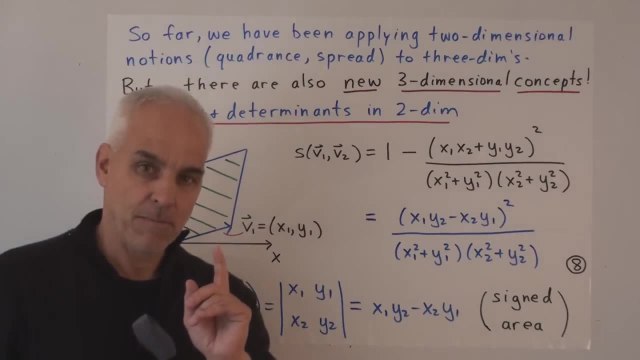 dot, product squared divided by the quadrants of V, 1 times the quadrants of v2. now we saw last time that, because of Fibonacci's identity, we could in fact rewrite this expression- in fact it's somewhat more compactly in this way. I didn't actually write down this. 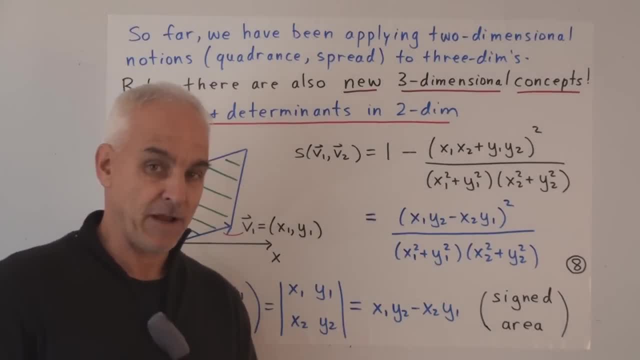 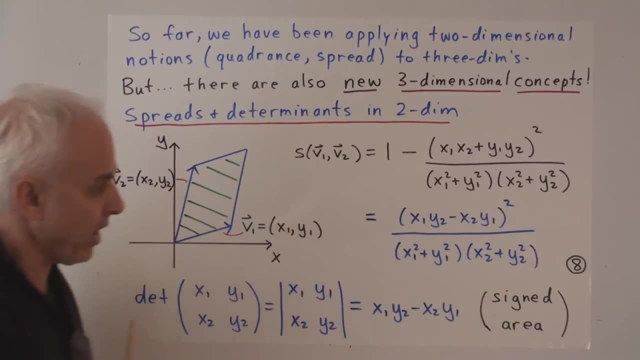 but it follows directly from the formula that I wrote down and I hope you discovered this while you were doing one of those exercises. The spread can be written in this more compact way, where the numerator now is x1y2 minus x2y1, all squared. 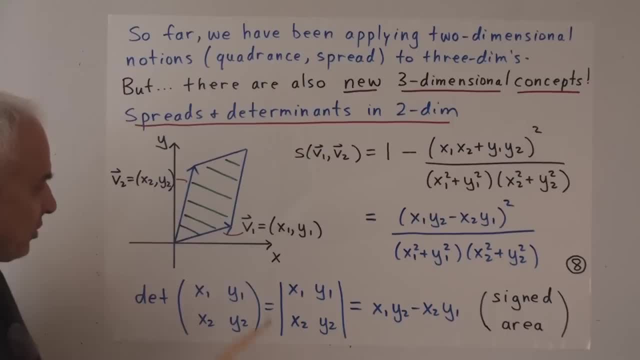 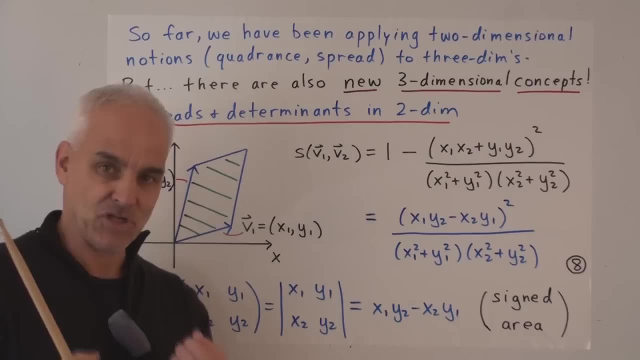 This expression is exactly the quantity that we need to check whether v1 and v2 are parallel. Remember, this was exactly the condition that v1 and v2 are parallel. when this quantity is zero, This quantity here, of course, is also a determinant. 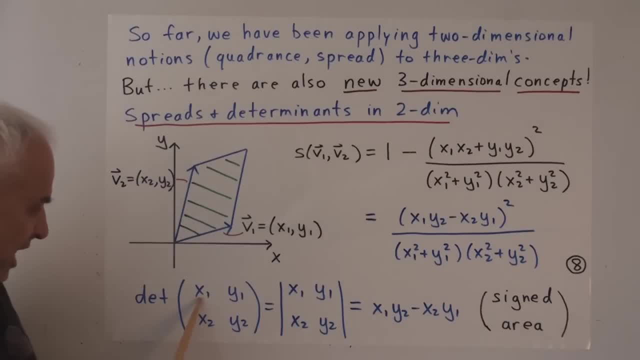 So in linear algebra, if you make a 2 by 2 matrix which has the first row the coefficients of v1, and the second row the coefficients of v2, this determinant, which is often written with a straight line bar there. 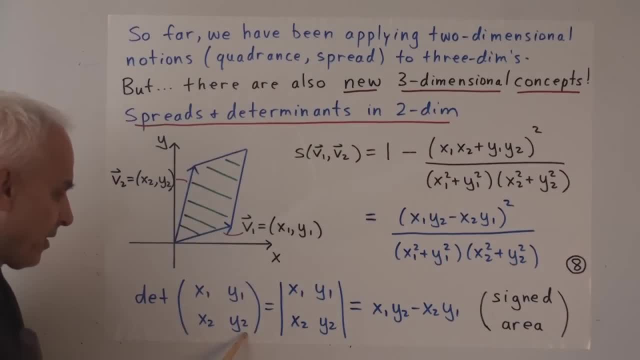 that has the value x1y2 minus x2y2.. That's 2y1.. That's the definition of a 2 by 2 determinant And in two-dimensional geometry, that's the signed area of the parallelogram formed by v1 and v2.. 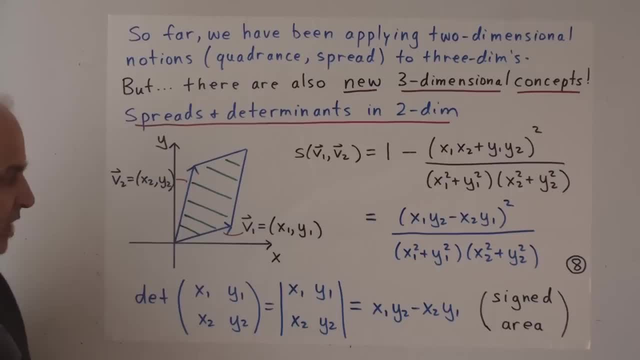 So these two vectors form a parallelogram, a very natural object in vector geometry, And the area of that parallelogram is given algebraically by this expression. So a determinant area of a parallelogram. pretty well the same thing. 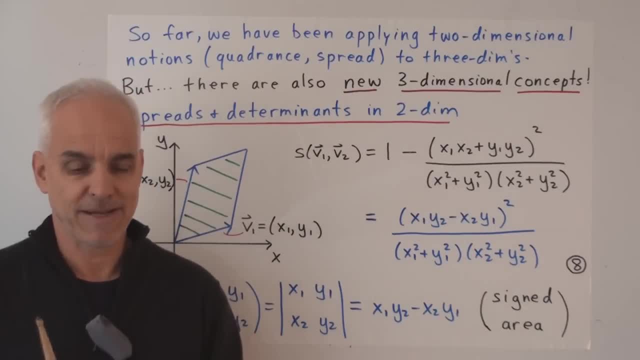 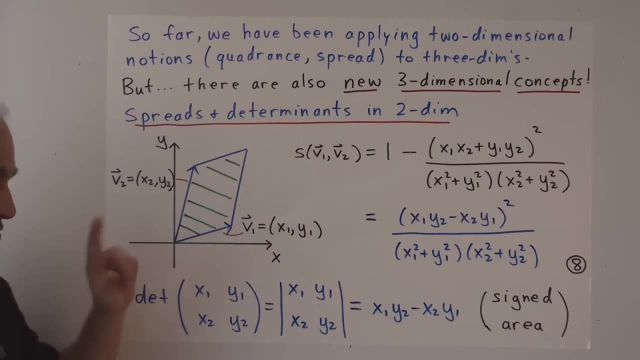 It's one of the reasons why the determinant is so important, because it encodes areas. Actually, it's a signed area in the sense that if you interchange the order of v1 and v2, then the determinant changes sign. What's happening in this expression is that the determinant is being squared. 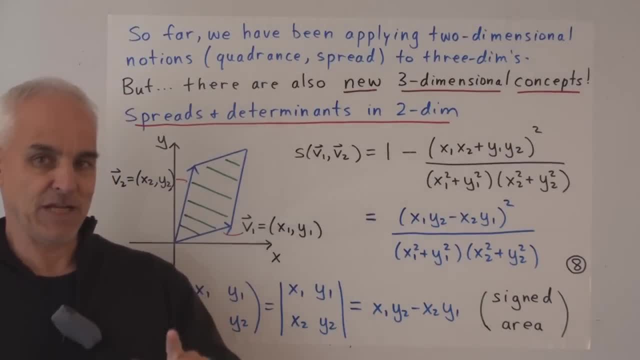 So that changing of sign that occurs when you interchange v1 and v2, becomes irrelevant, Because even if the sign inside changes when you square it, nothing changes. So how should you think of this? You should think of this as some kind of normalized area. 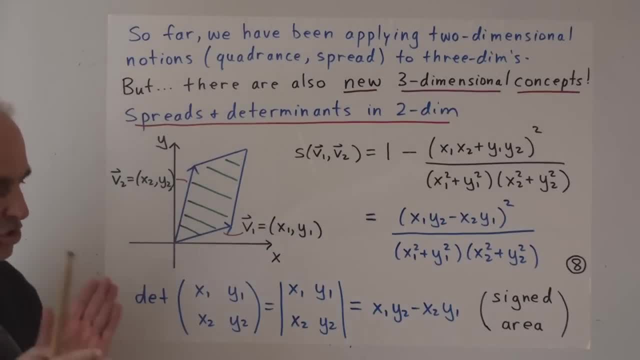 We're taking the area of this parallelogram, we're squaring it and we're dividing by the quadrants of this times, the quadrants of this. That means that it's an object which is scale independent. It doesn't matter what the notion of scale is on the axes. 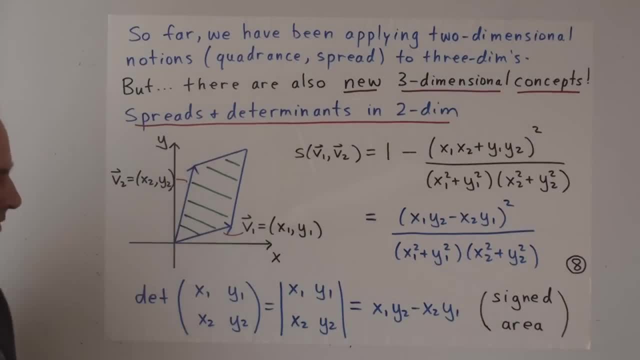 So I haven't actually put any scaling on these axes, you've noticed. So, although without a sense of scale you can't really say what the area is, but you can say what this normalized sort of squared area area is: This quotient between the square of the area and the product of the quadrants. 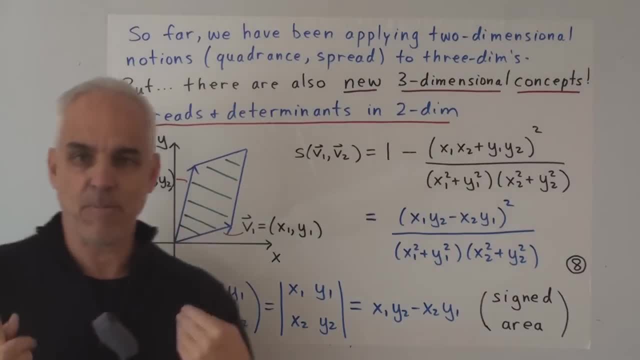 is, that's the spread between the two vectors that is independent of scaling. This is another way of thinking about what the spread means. It's some kind of area or normalized area contained between the two vectors. It's a very important additional way of thinking. 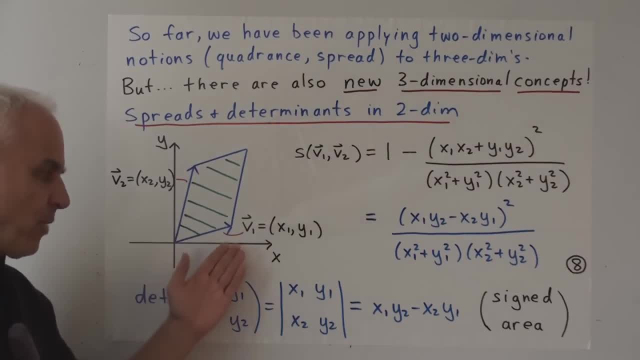 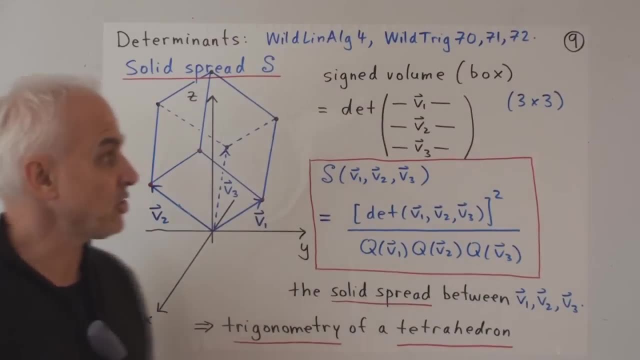 about it. So let's have a look at what this approach looks like in three dimensions. So if you'd like to have a bit of review on determinants, I suggest my Wildland Algae 4 lecture and also the Wild Trig lectures 70, 71 and 72.. It's also a bit of discussion of determinants there. 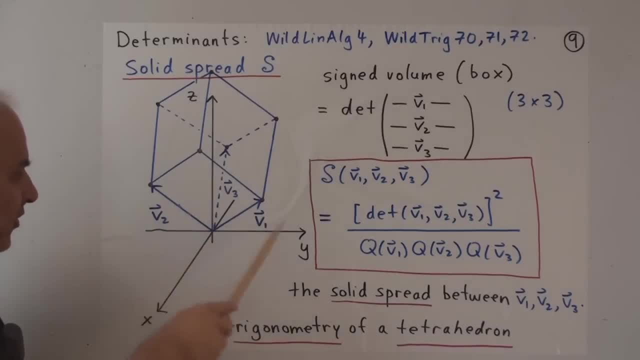 Alright. so here we're jacking things up to three dimensions. We have now our x, y, z coordinates, And now we have three vectors: v1, v2, and v3.. And just as two vectors in the plane form a parallelogram, so do three vectors in space form a parallelepiped, which is a box. It's. 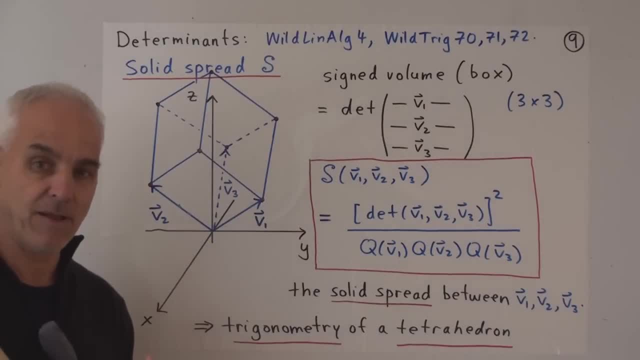 a box whose sides are all exactly parallel and equal to the three vectors. So this vector and this vector, and this vector and this vector are all the same, And this one, this one, this one and this one are all the same. 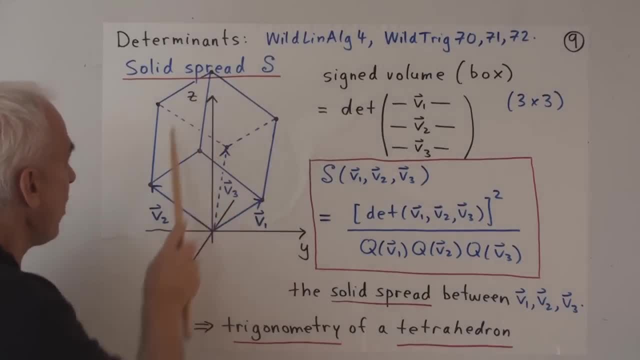 And this one, this one, this one and this one are all the same. So the front and the back sides of the box, or this one and the other side, or the bottom and the top, those sides in pairs are all exactly identical And the way I've drawn it here, 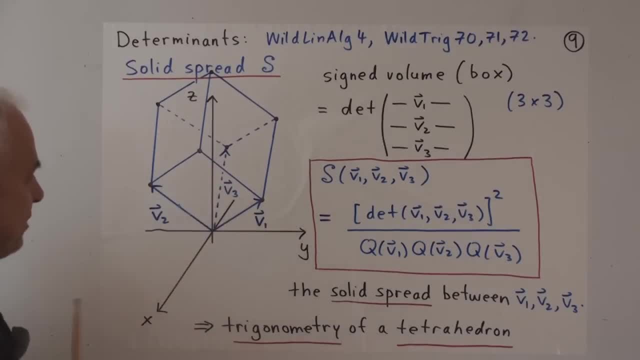 you're supposed to think of this V3 vector as sort of being behind. So V1 and V2 are closer to you and V3 is sort of behind, So hence the dotted lines. The three-dimensional aspect of the box is a little bit indeterminate. Sometimes you might see this point as being 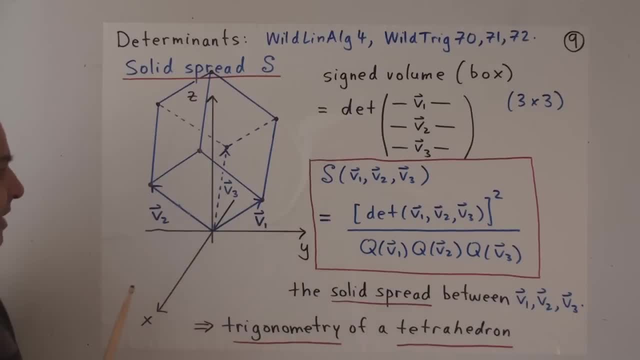 the point in the box that's closer to you, and if you look at it again a minute later, you might find this point as suddenly being the point that's closest to you and this one sort of at the back. They can often sort of switch back and forth. 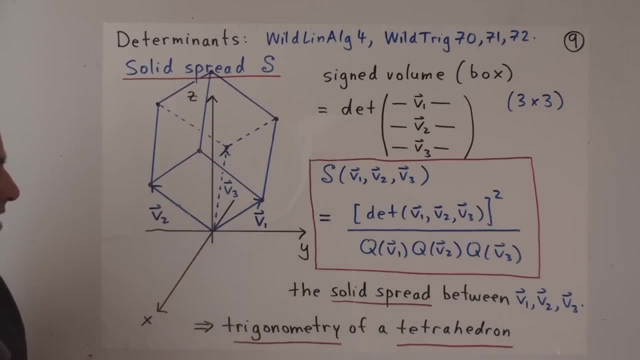 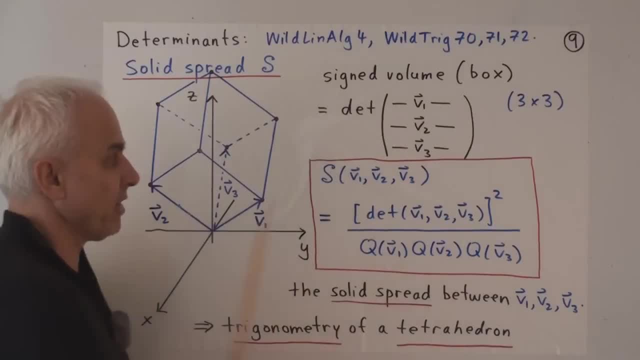 is a purely algebraic thing in terms of a determinant. It's the determinant of a 3x3 matrix whose rows are the coefficients of the three vectors. So V1 along the top row, V2 along the second row, V3 along the third row. That's a 3x3 matrix, and if you take 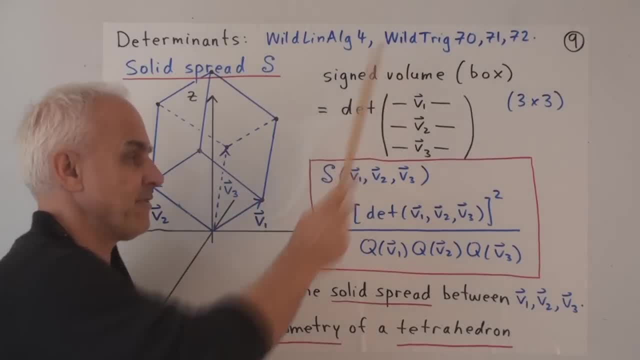 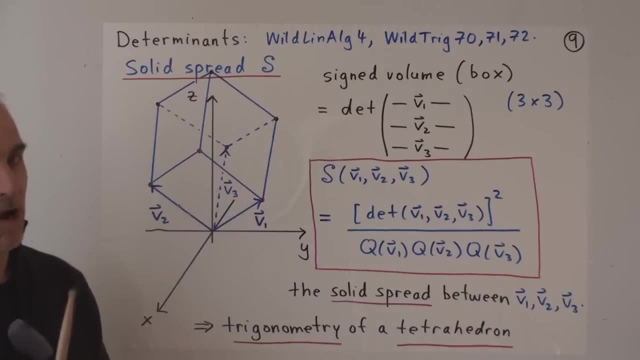 its determinant- and you can review what that means from these videos- then that determinant represents the volume of that parallelepiped or box, And it's also a sine volume, strictly speaking. Sometimes it can be negative. One of the properties of the determinant is that if you 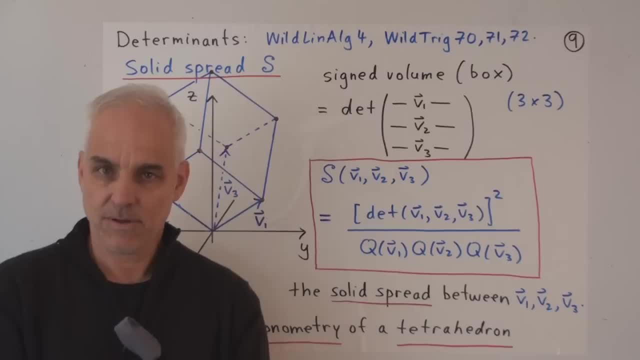 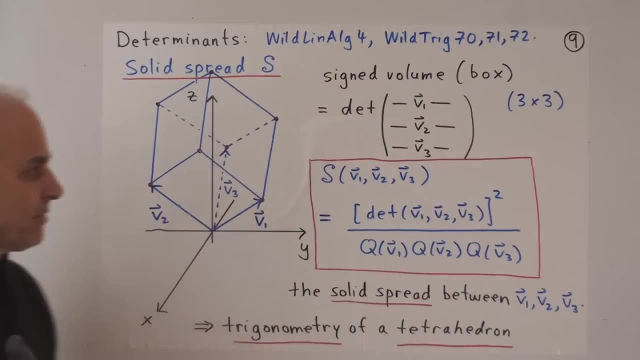 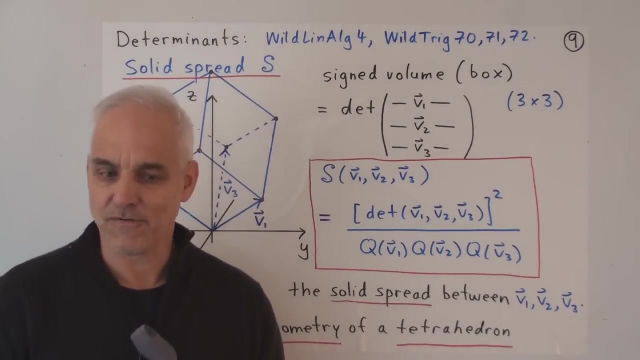 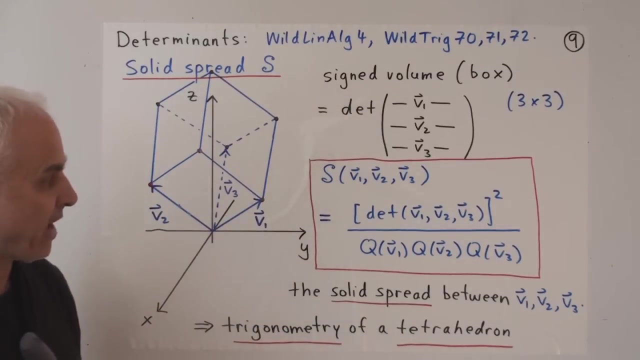 interchange any two rows, the determinant changes sine. So it's sensitive to orientation. so it's sensitive to orientation, All right. so exactly analogous to the second formula for the spread of two vectors that we had in our previous slide, we're now going to introduce a concept that measures how far 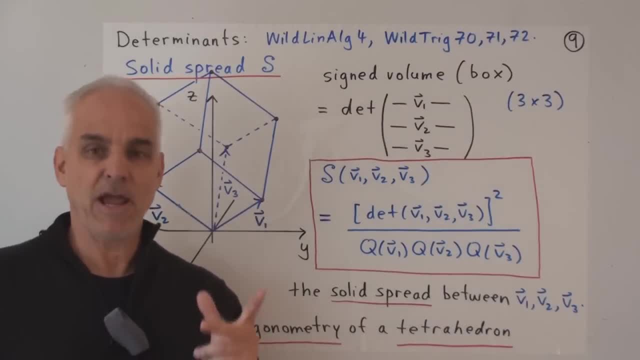 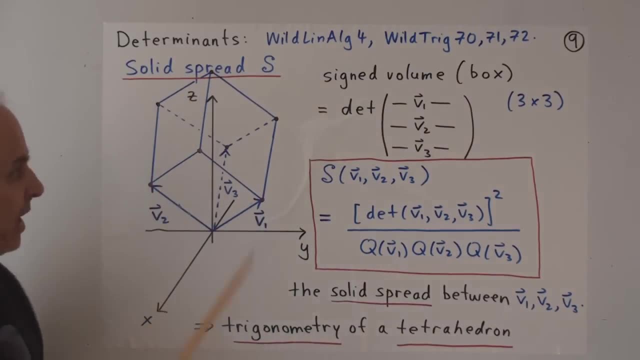 these three vectors are apart, The spread between three vectors. We're going to call this a solid spread And we'll denote it by a solid spread. And we'll denote it by a solid spread And we'll denote it by a sort of curly or calligraphic S. So the solid spread between V1, V2,. 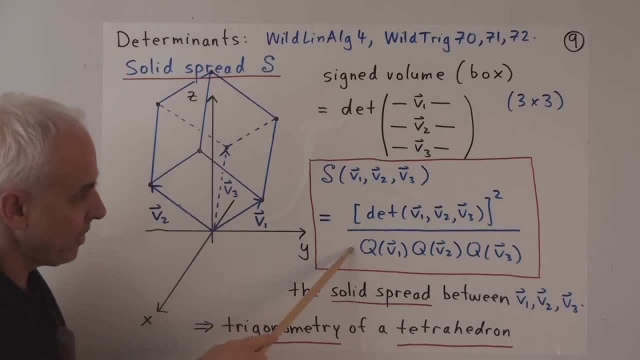 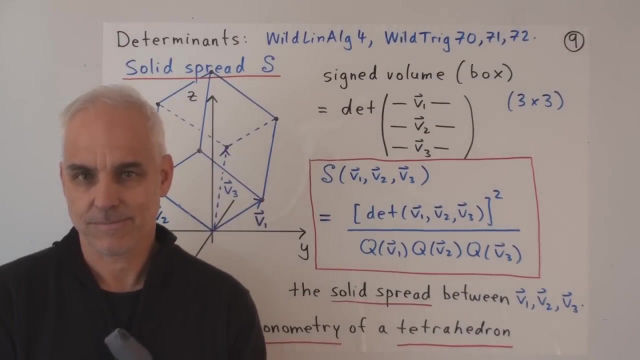 and V3 is the quotient of this determinant squared divided by the quadrants of V1 times the quadrants of V2, times the quadrants of V3. So this turns out to be a three-dimensional analog of the spread, And it's rather important for three-dimensional 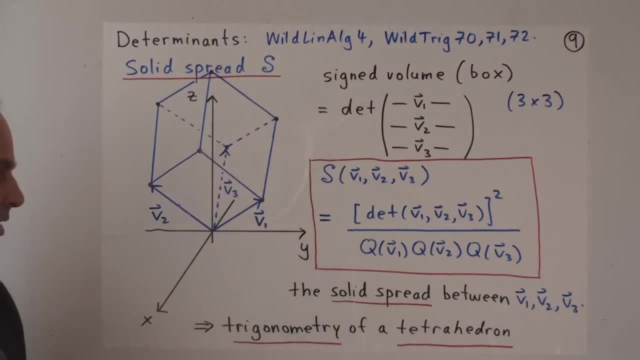 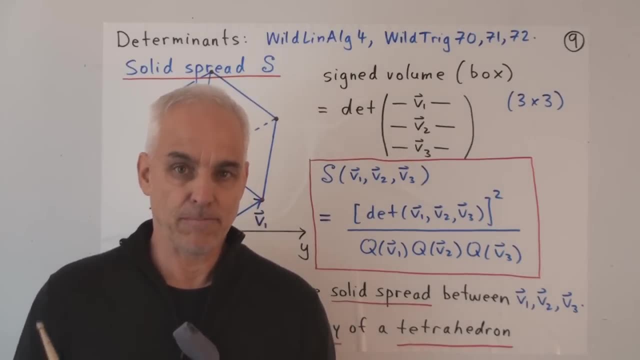 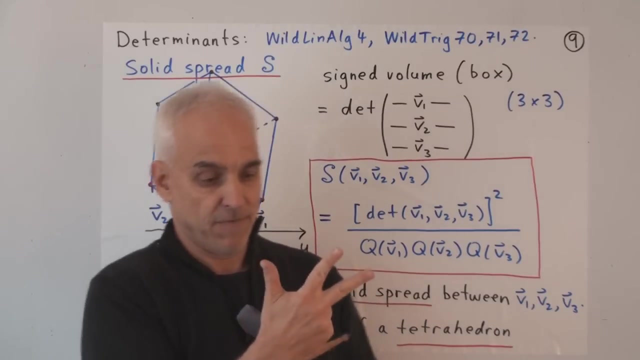 trigonometry and geometry, as we'll see later on. So it turns out that when you have this distance angle orientation, as do most modern mathematicians, then three-dimensional geometry becomes very hard to work with. The formulas become very complicated. The angles, especially, doom you to making everything complicated. In the planar case, if you have three lines which are planar, 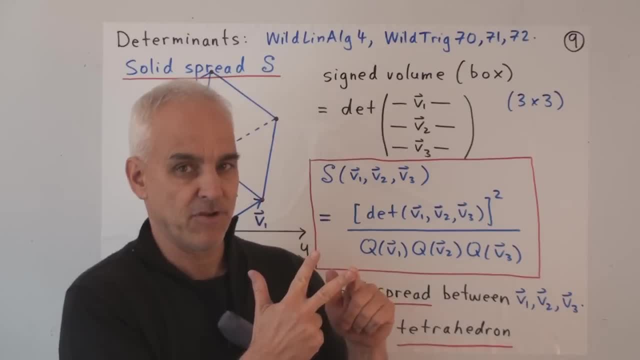 you can at least say that this angle of five degrees and this angle of seven degrees is a total angle of twelve degrees. It'll give you a little bit of a psychological boost. You think, oh, I'm doing geometry. Five plus seven is twelve. 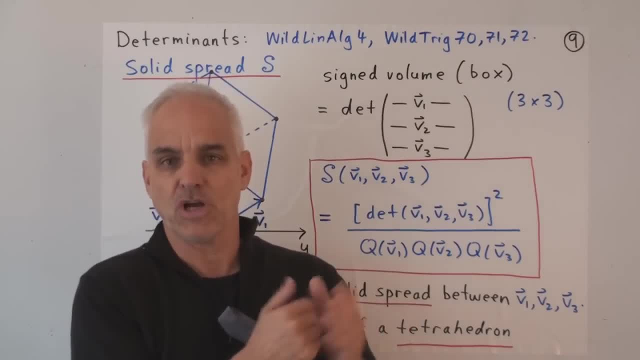 And many people think this is good for young children to learn because they're learning geometry. It's actually a waste of time. largely It's because the angle, this seeming linearity, is an artificial linearity And you impose it and you may force it on the structure, but it doesn't want to be there. 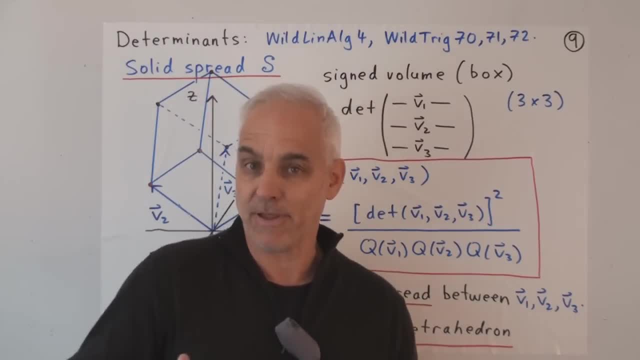 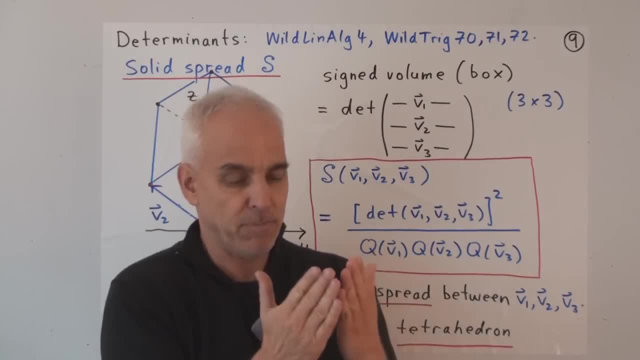 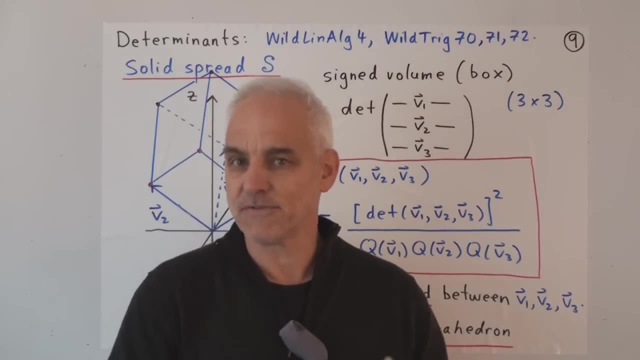 one angle in one plane and then another angle in another plane and the two planes are at some angle. well then things get very complicated. You have to essentially use the laws of spherical trigonometry even to add the angles. It's rather interesting that even undergraduate students who graduate with a degree in mathematics, 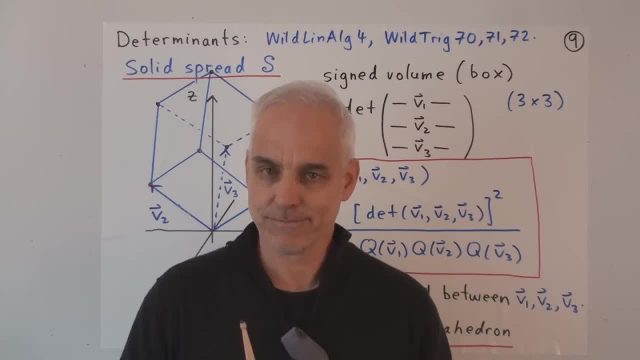 their understanding of three-dimensional space is pretty minimal, And this is surprising, Since we live in three-dimensional space and you would expect mathematics to be pretty well on top of describing very clearly and effectively what goes on in this three-dimensional space. So one of the advantages in the rational trigonometry point of view is that we can really get our hands on three-dimensional geometry. 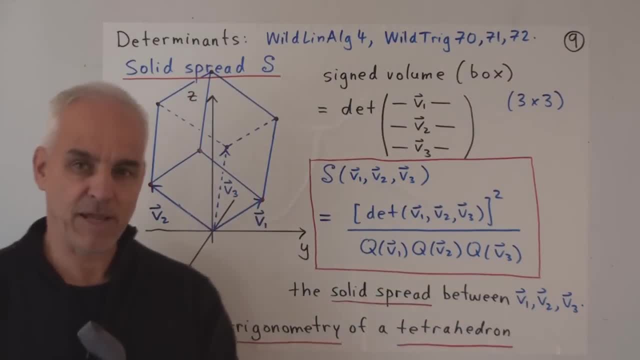 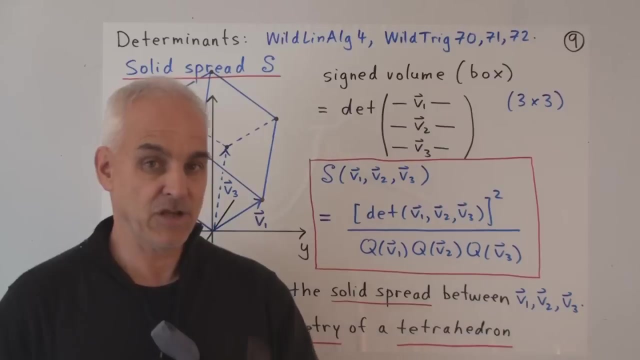 And it will turn out that the trigonometry of a tetrahedron plays the critical role. Just as a triangle is critical in two dimensions, so the tetrahedron is crucial in three dimensions. And with classical trigonometry, figuring out what goes on in even a tetrahedron is a major challenge. 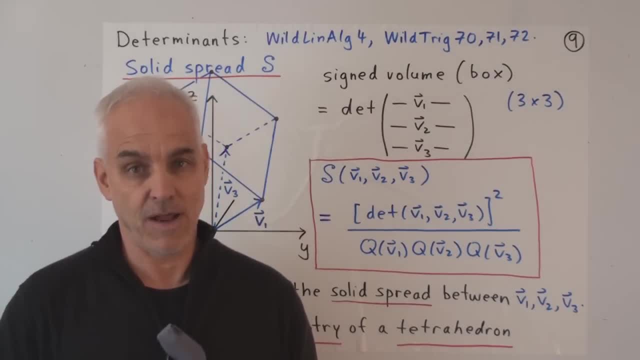 which has not been, as far as I understand, properly done. We are going to be able to understand a tetrahedron properly in the fullness of time. I may actually do that in my Wild Trig series. It probably belongs more properly there. 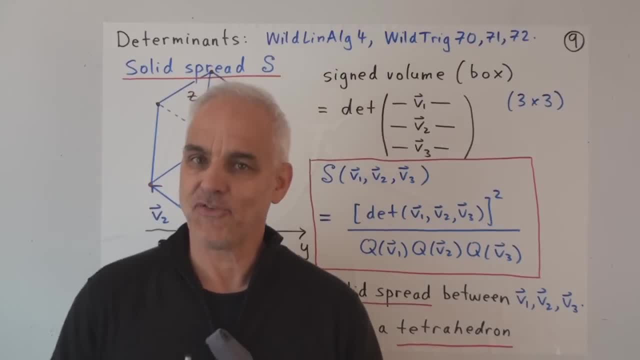 But some of it will also be filtering through to this course in hyperbolic geometry. Alright, so we have enough foundations now for three-dimensional geometry and trigonometry that we can turn our attention to the sphere and elliptic geometry. So next time we are going to introduce the basics of trigonometry in the elliptic geometry setting. 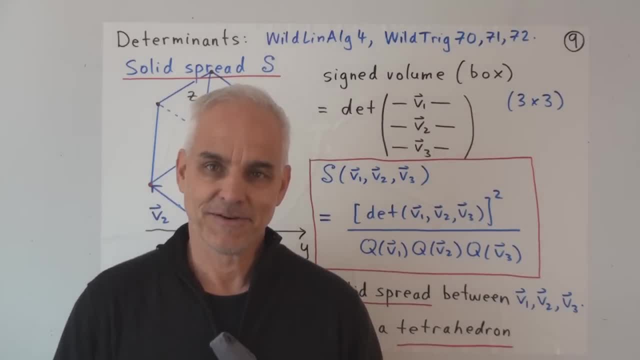 I hope you will join me for that. I am Norman Walberger. Thanks for listening.